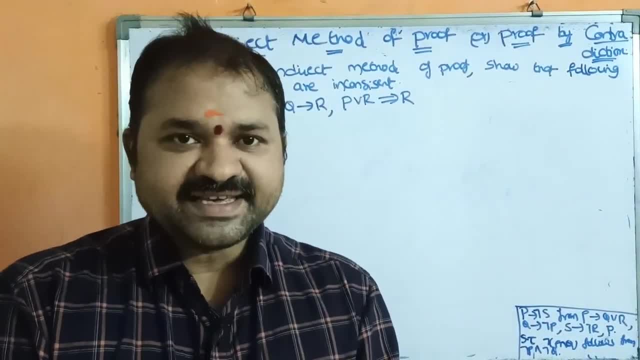 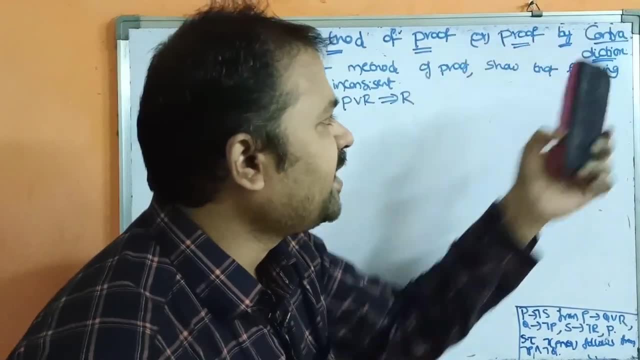 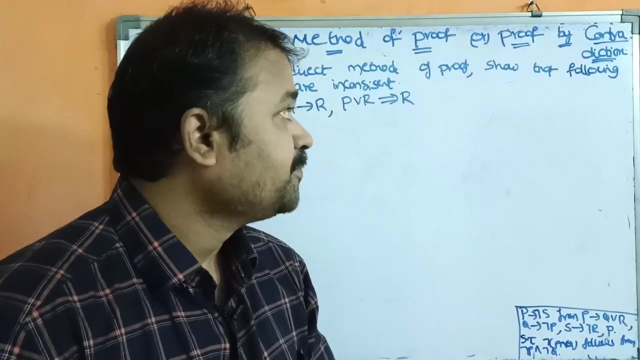 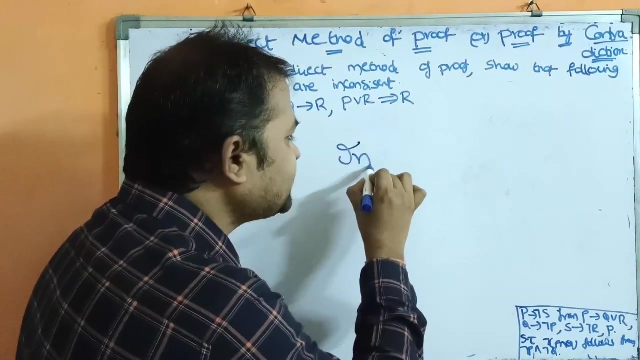 In this video we are going to discuss about indirect method of proof or proof by contradiction. First let us see what is the use of indirect method of proof or proof by contradiction. It is mainly useful in order to check whether the premises are inconsistent or not. So by 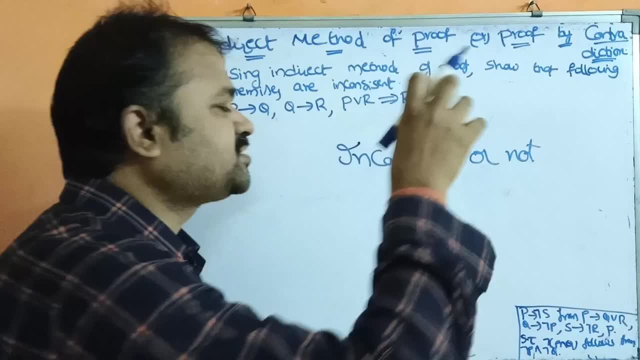 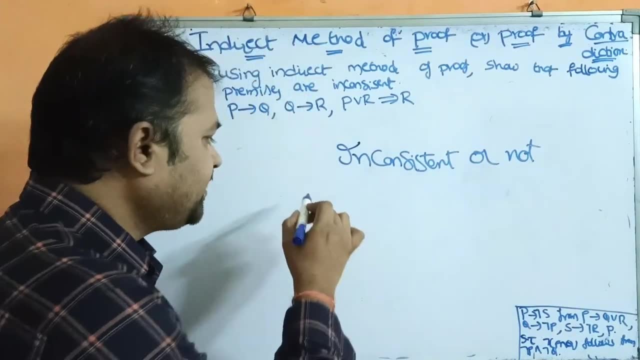 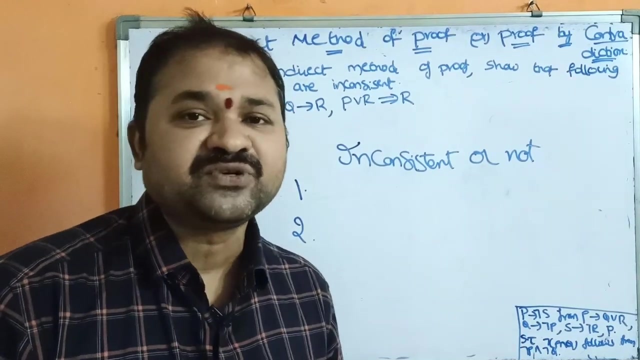 using indirect method of proof. mainly, we prove that the premises are inconsistent. Let us see how we can do that Here. there are two steps, are there? Let us see those two steps. The first step is we have to introduce negation of the conclusion. Let the conclusion 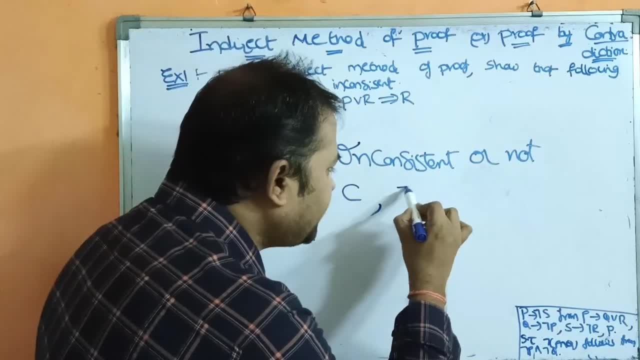 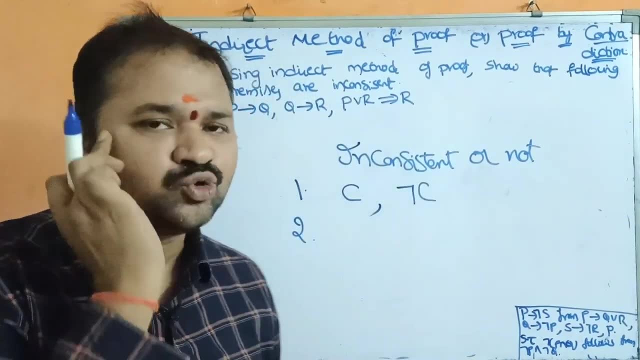 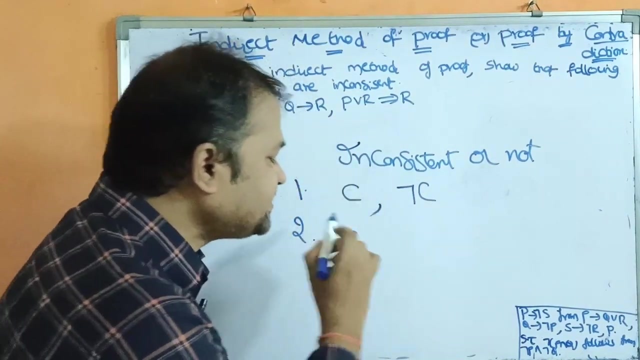 is C, Then we have to introduce negation of C. Next we have to add negation of C to the existing premises And the second step is if the new premise that is negation C with the existing premises, that means with the given premises. 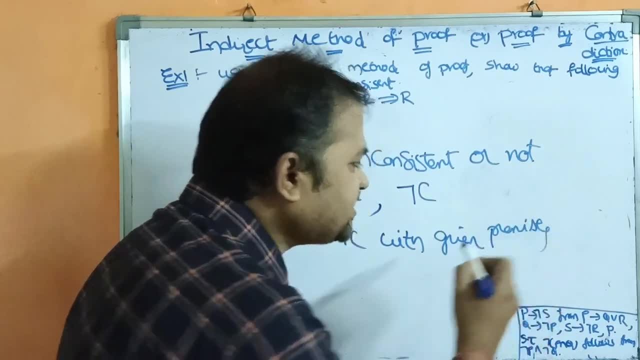 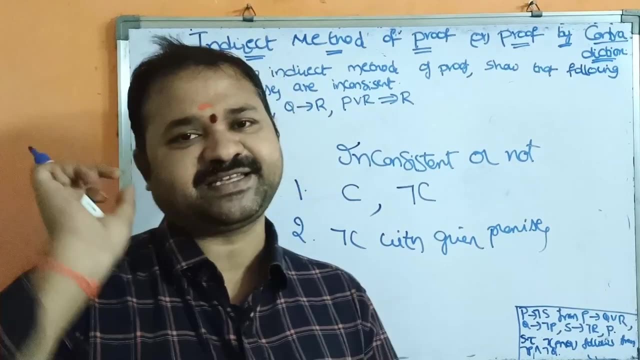 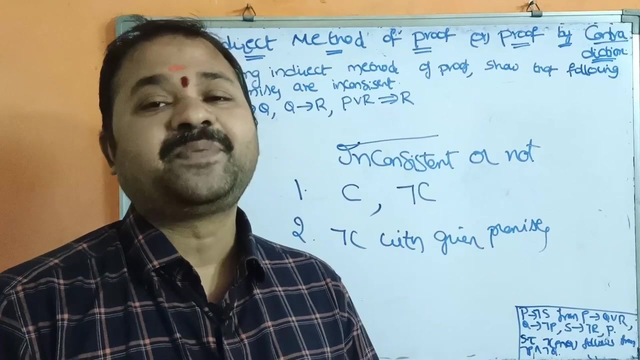 produces a contradiction- Contradiction means false- Then we can say that those premises are inconsistent. Let us see that one more time. So by using indirect method of proof mainly, we prove that the premises are inconsistent. Indirect method of proof can also be called. 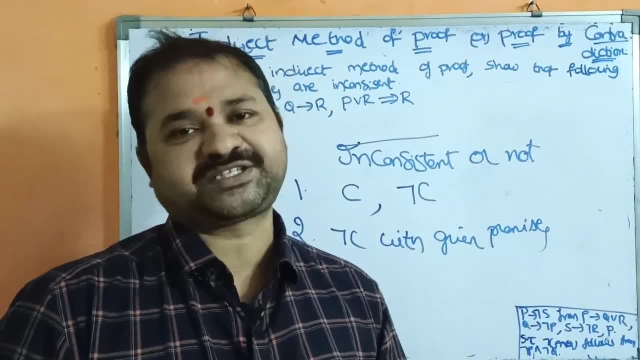 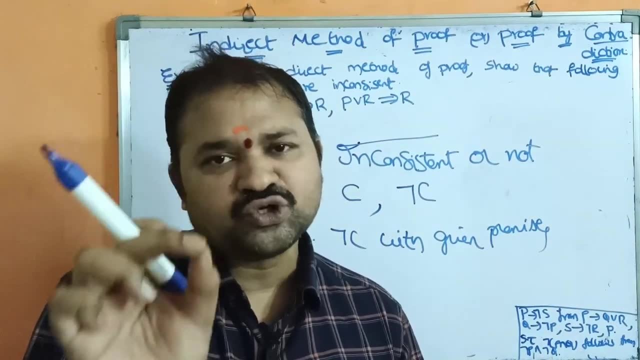 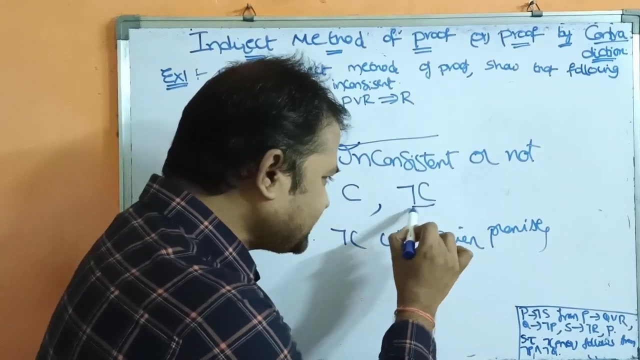 as proof by contradiction. Contradiction means false. Here we have two steps, are there? The first step is we have to introduce negation of the conclusion to the given premises. So let the conclusion is C, Then what is the negation of the conclusion? Negation C, So. 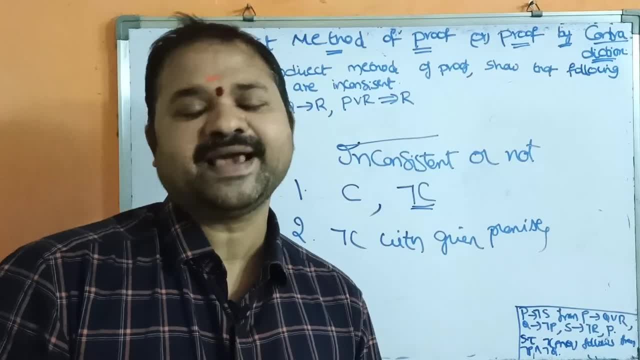 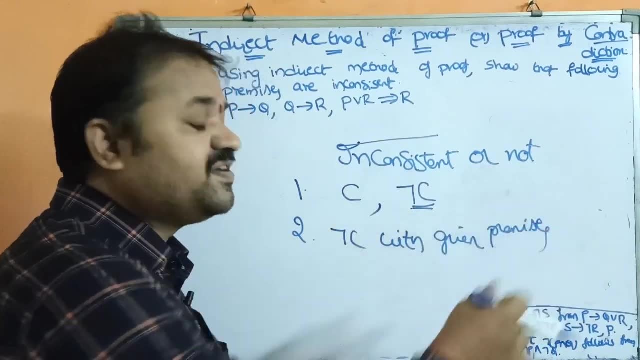 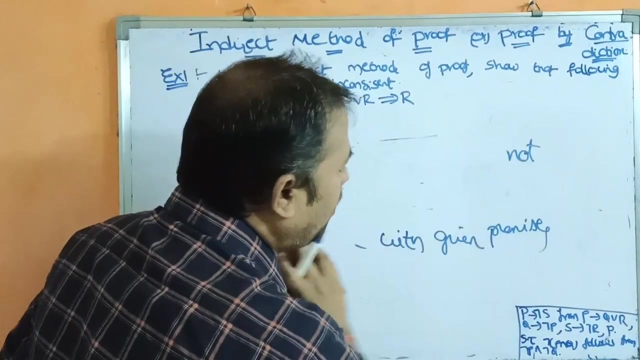 we have to add this premise to the existing premises. So let us see how we can do that premises. and the second step is that that that new premise with the given premises produces a contradiction- false. then we can say that the premises are inconsistent. so let us solve three. 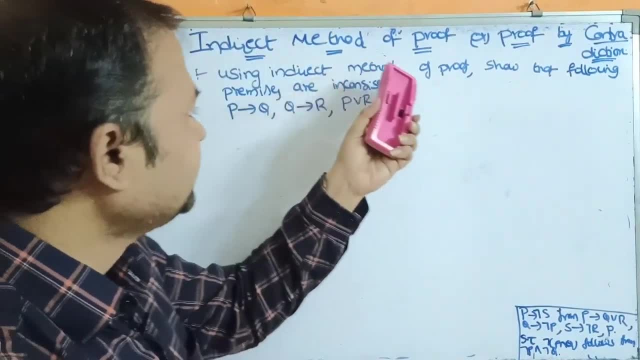 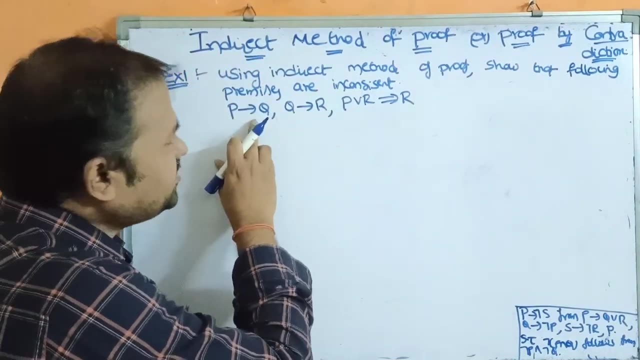 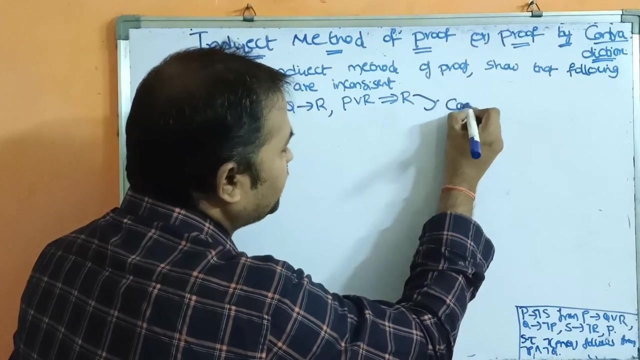 examples in this video. let us see the first example using indirect method of proof. show that the following premises are consistent. so p conditional, q, q conditional or p conditional, or implies r. so that means this: r here is conclusion. so what is the negation of the conclusion? 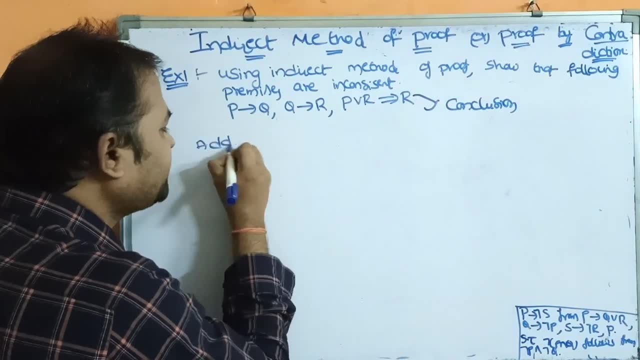 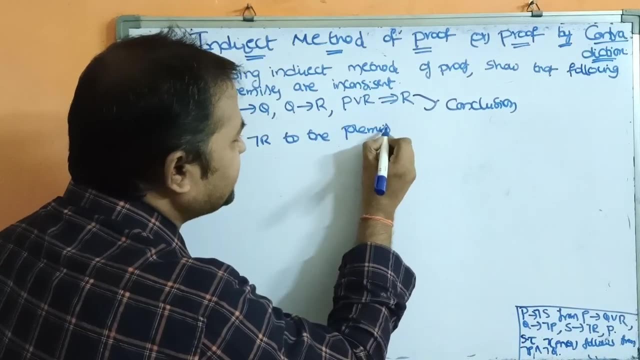 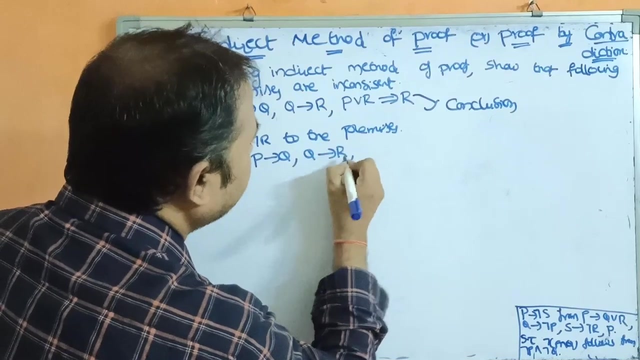 what is the add negation of the conclusion? so you add negation r to the premises. so we have to add negation r to the premises. so the given premises are p, p, conditional, q, q, conditional r, p, r, r, as well as negation r. okay, this negation r is the new new. 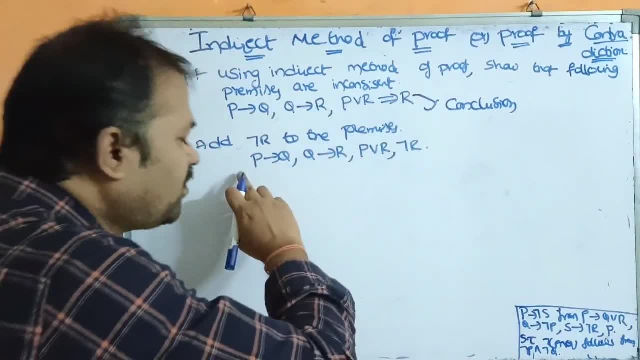 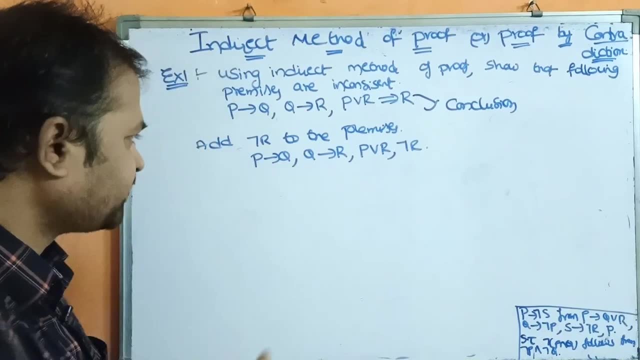 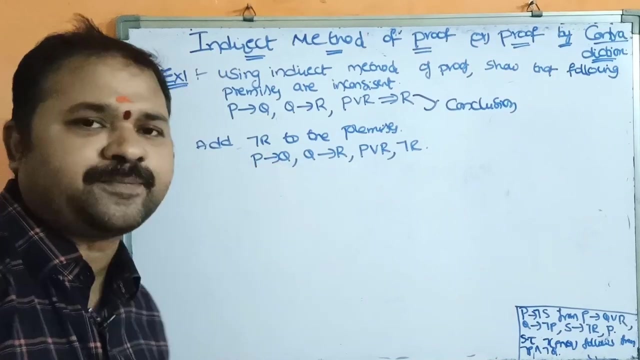 premise that negation of the conclusion. so by using all these premises, if we get the result as false, then we can say that the premises are inconsistent. okay, let us observe here: here we have p conditional q, here we have q conditional r. so from this we will get p conditional r. so let 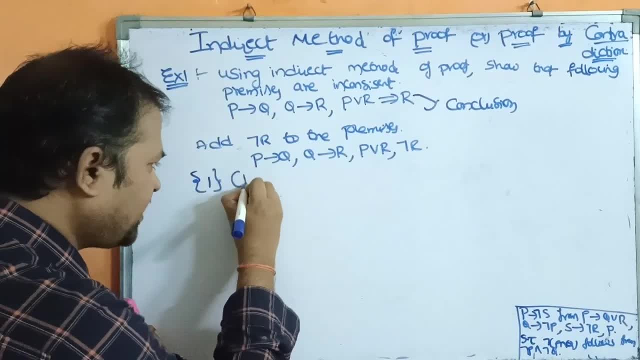 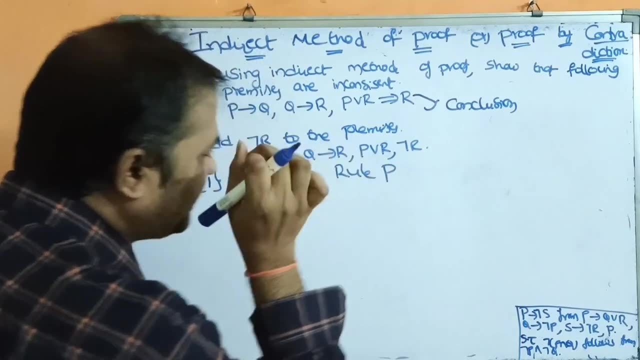 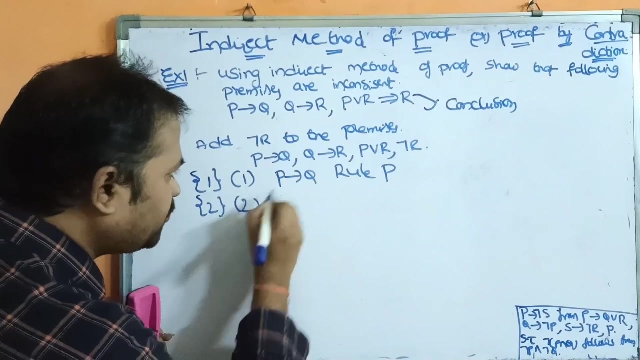 us see that. so first to premise. so formula number is one. let us introduce p, conditional q. so this is p premise. in the derivation process it is called as rule p. now let us introduce the second premise. this is formula number two. what is the second premise? q conditional r. and here we need: 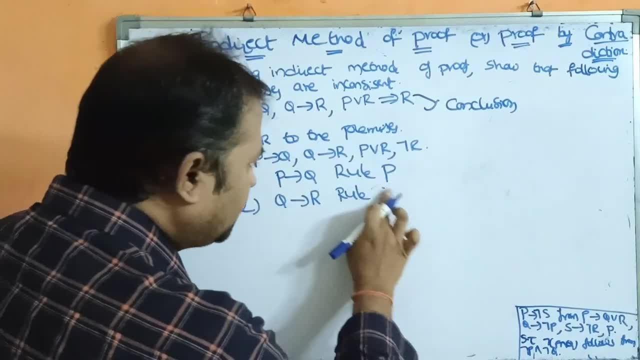 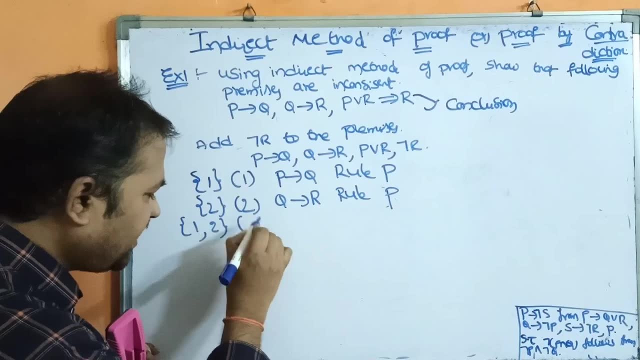 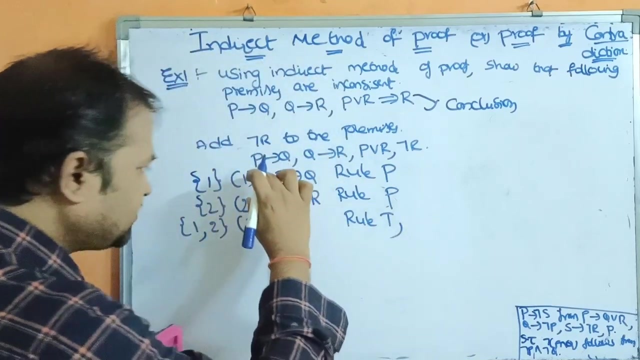 to apply rule t, on which this is. first we have to introduce the premise, so this is also rule p. next, based on first premise and second premise, we are deriving the new formula. so one and two is over, so the next formula is rule three. here we need to apply rule t, on which formula? 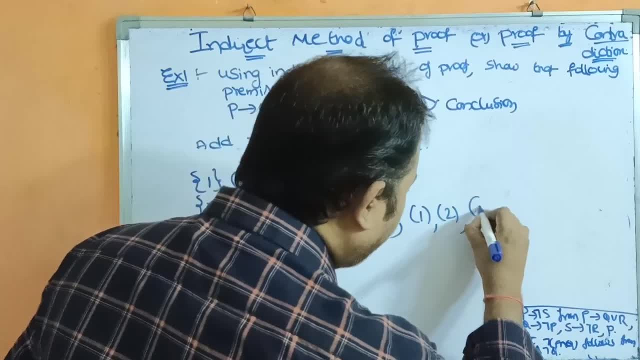 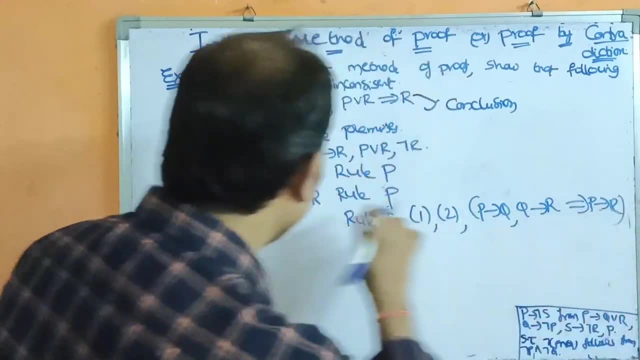 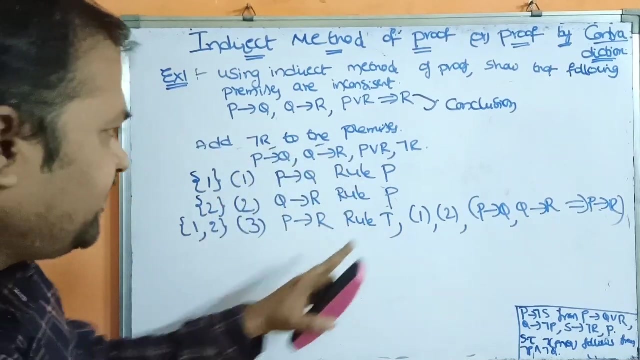 numbers on one and two and which formula we have to apply. p conditional q comma. q conditional r implies p conditional r. okay, so p conditional q, q conditional r means what? p conditional r? so these two premises are taken. so here we have negation r. so let us introduce that premise we, so that we: 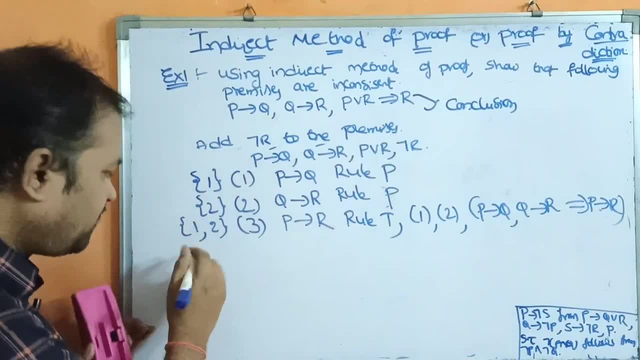 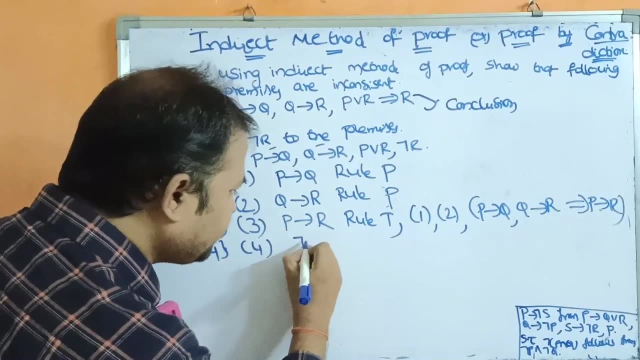 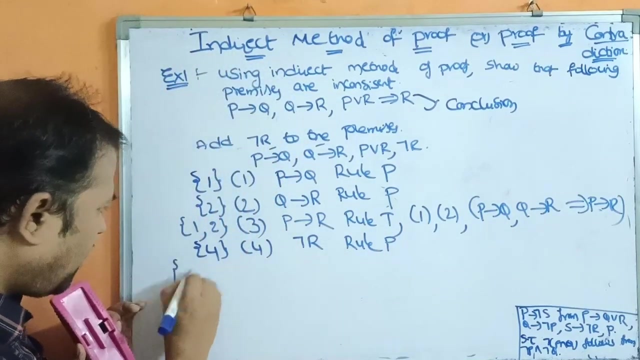 can cancel r and negation r, we will get p, okay. so first let us introduce negation r. so formula number is three is over. so next premise: number is four, four. here we are introducing negation r, here we are introducing this premise. so this is nothing but rule p. now let us apply the formula on these two premises. so one comma two. 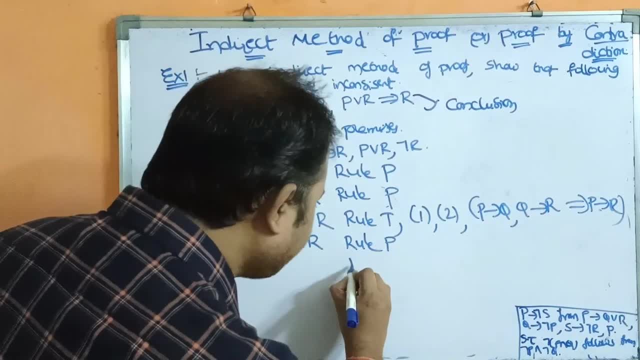 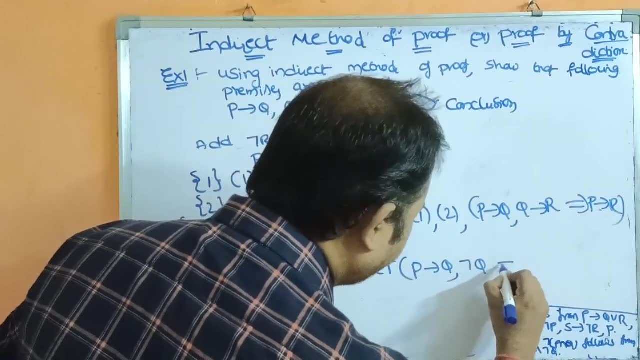 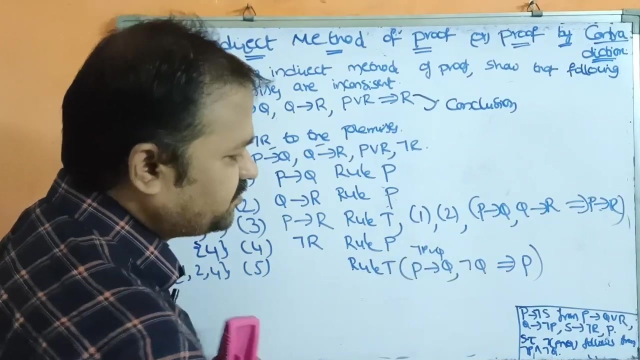 comma four. next formula number is five here. what is the rule? we are applying? rule t. here we have a rule called p implies q comma. negation q implies p. why? because p implies q means what negation p? rq. here we have negation q so we can cancel q or negation q, so we will get this negation p. i am sorry, we will get negation p as. 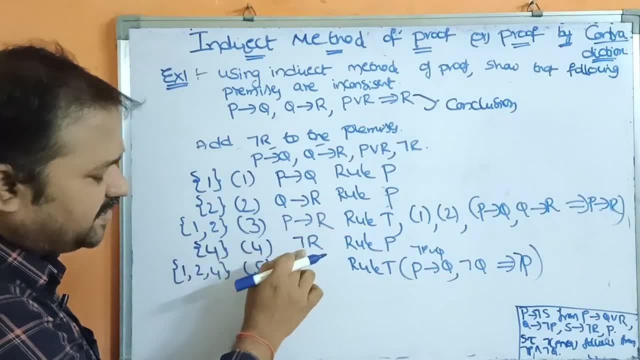 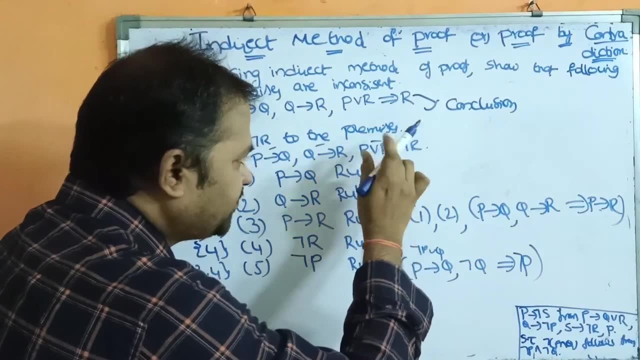 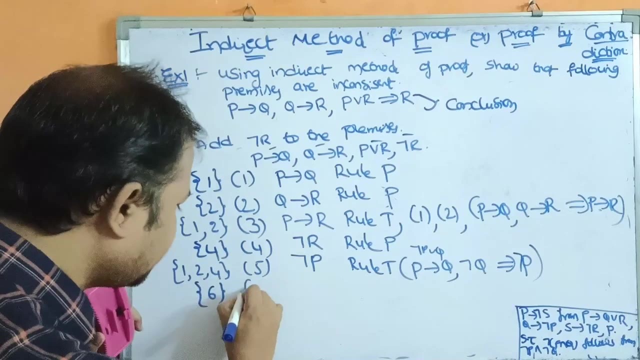 the result. so if you take this one, so negation p rr, negation r, we can cancel r and negation r, so we will get negation p as the result. okay, so this premise is also taken. so the last premise is p- rr. let us introduce that premise. so formula number five is over. so the next premise is six formula. 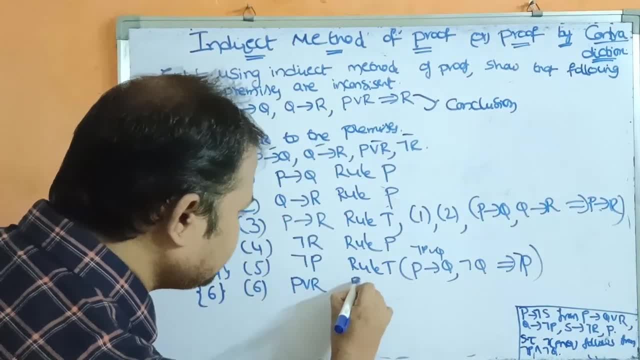 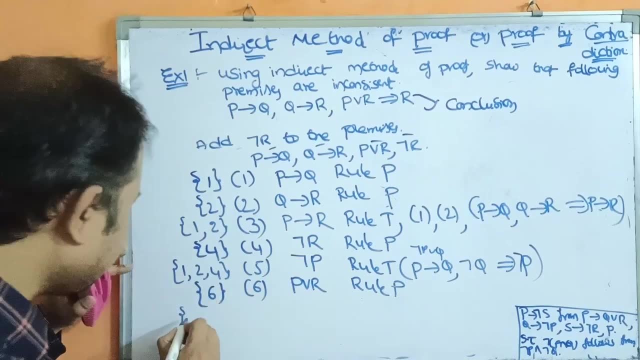 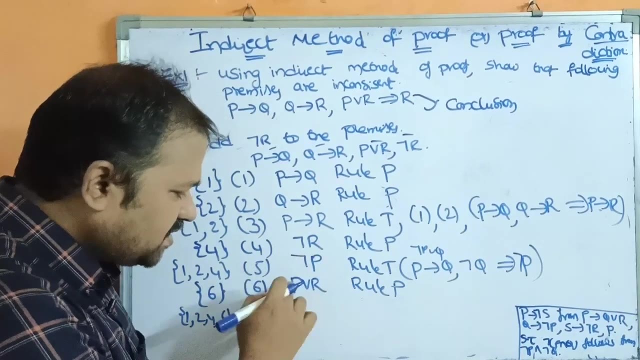 number is six. so let us introduce p? rr. so this is nothing but rule p. why? because introduction of the premise. okay, so next we have to apply the formula on these two premises. so one comma two, comma four, comma six. next formula number is seven. here we have negation p pr? r, so we can. 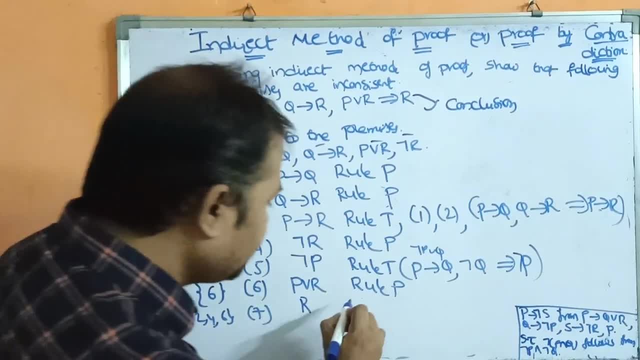 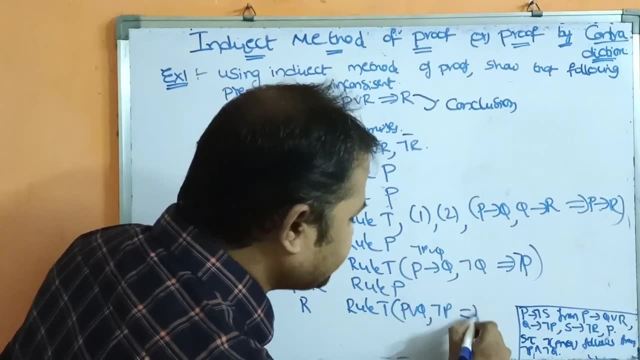 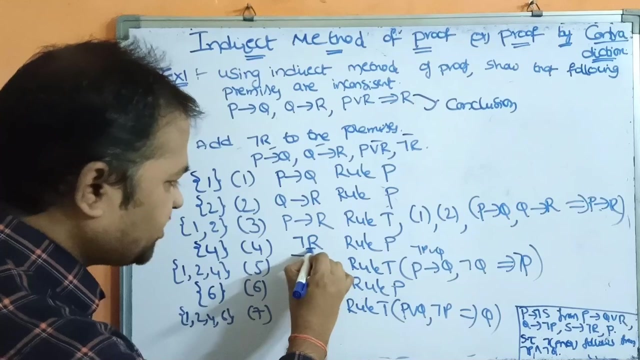 cancel p and negation p, so we will get r as the result. okay, so this is nothing but rule t. so what is the formula? we have p r q comma. negation p implies we can cancel p and negation p, so we will get q here. okay, so here we have r, here we have negation r. we have a formula called if the 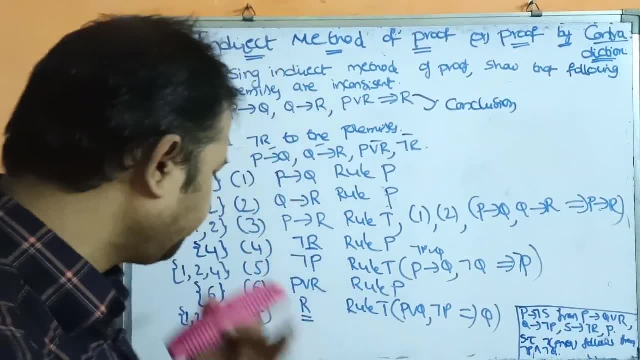 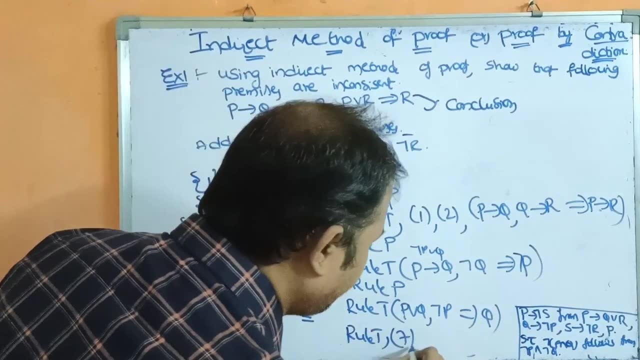 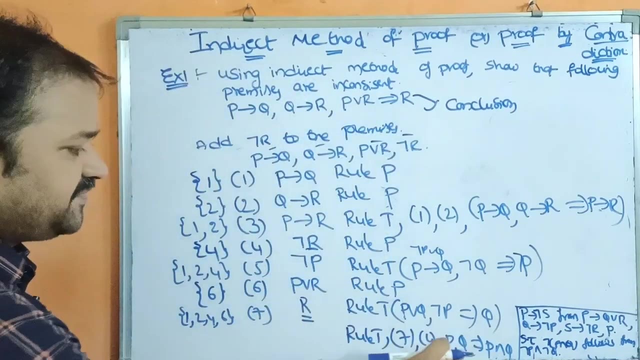 premises are p, q, then we can write as p and q. okay, so here we are applying rule t, rule t on which formula numbers on seventh one and fourth one, seven and four, or we can write as four and seven, there is no problem. p comma, q, conditional. if there are two premises like this, then we can write as p. 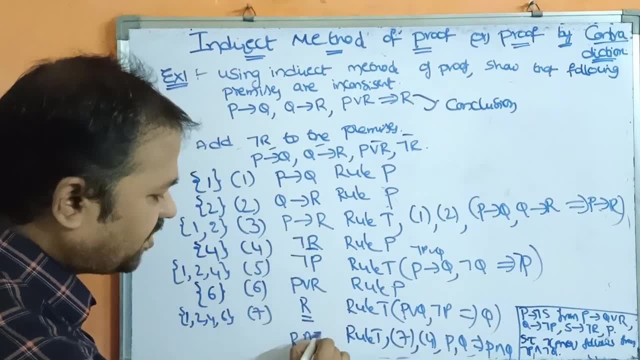 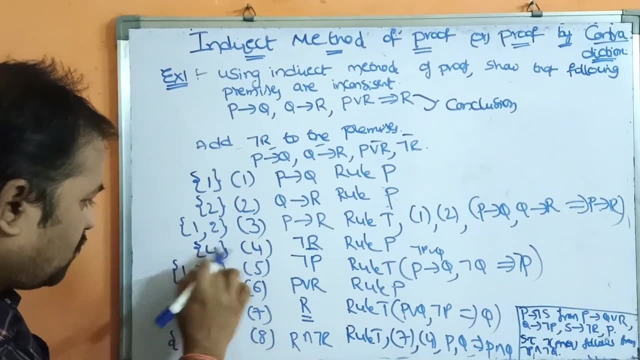 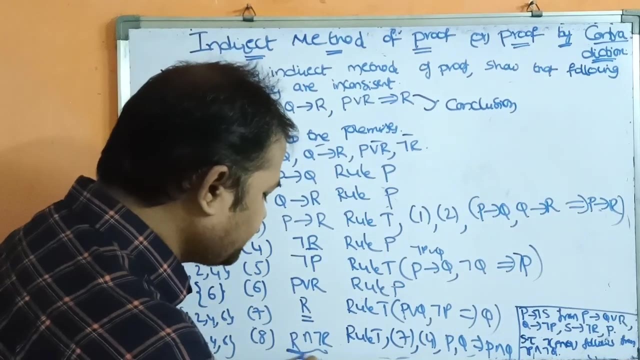 and q. here p means r and q means negation r. okay, you. so this is nothing but formula number eight. and here we applied on fourth formula and this fourth premise, and one, two, four, six. so one, two, four, six, repetition of four is not necessary. so r and negation r is nothing but what false. we have a formula called p and negation p is false. 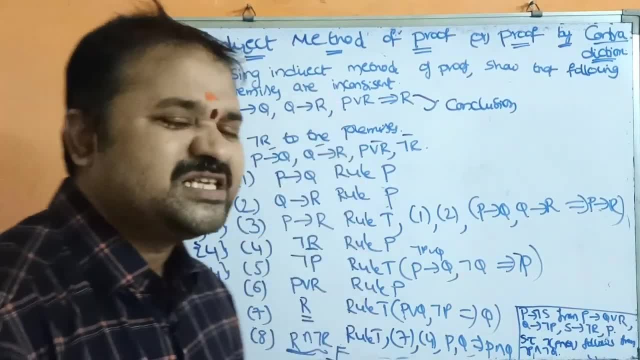 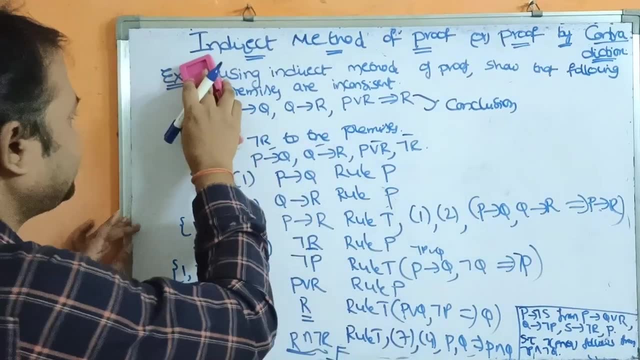 so we got false as the result, so we can say that all these premises are inconsistent. okay, if we got result as the false, then we can say that all these premises are inconsistent. let us solve the second example. so we have three examples, are there? let us solve those three examples. 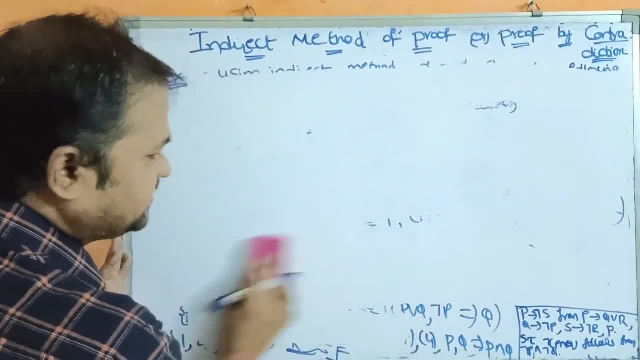 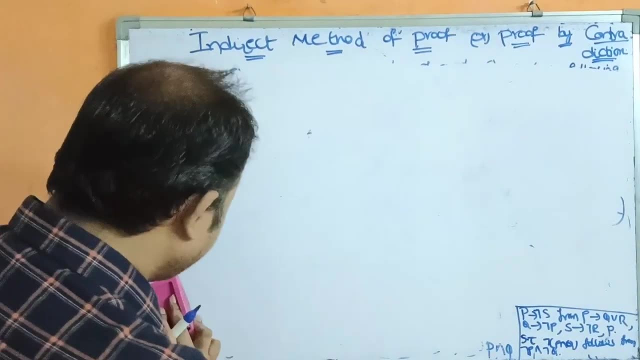 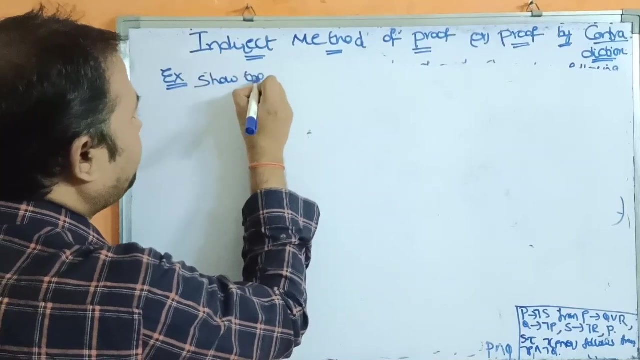 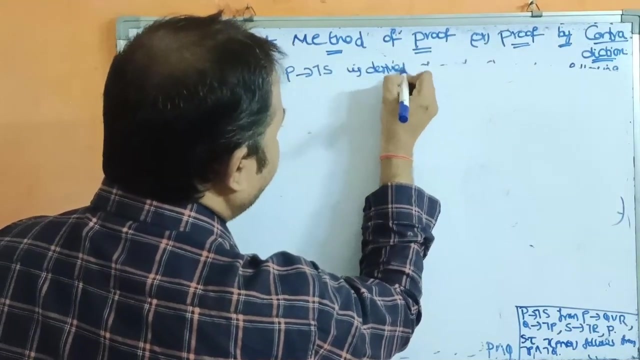 so if we, if we, if we solve these three examples, then you can solve any example which was which is given in the examination. okay, the second example is somewhat complex. here show that p implies negation yes. p implies negation, yes is derived from is derived from: 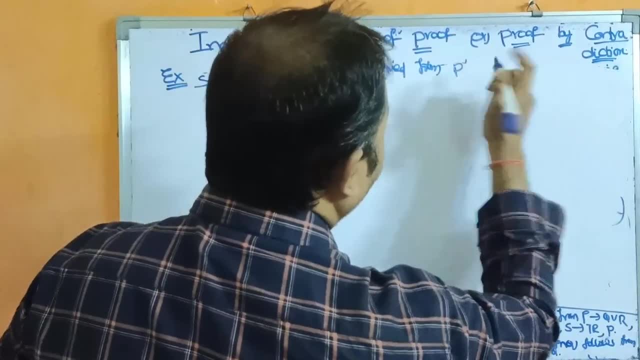 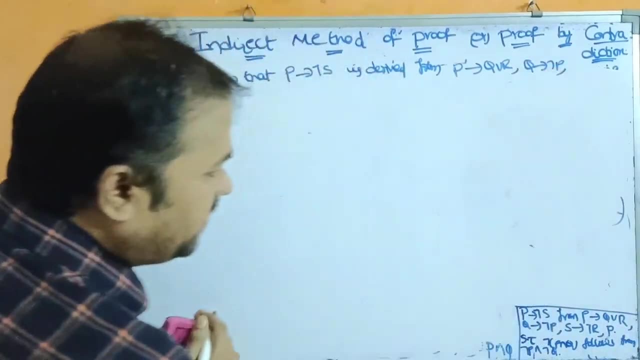 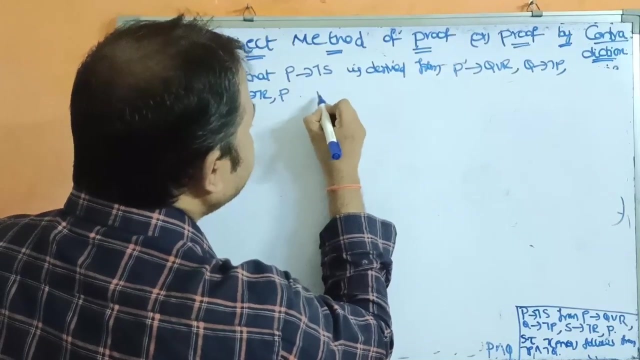 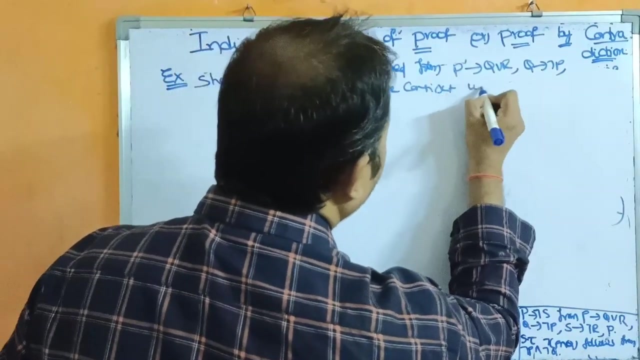 let us note the premises p, conditional p, conditional q, comma r, next to q, conditional negation p, comma s, conditional negation r, comma p. so we have to show that these premises are inconsistent. premises are inconsistent using which method? using con, using proof by contradiction. so proof. 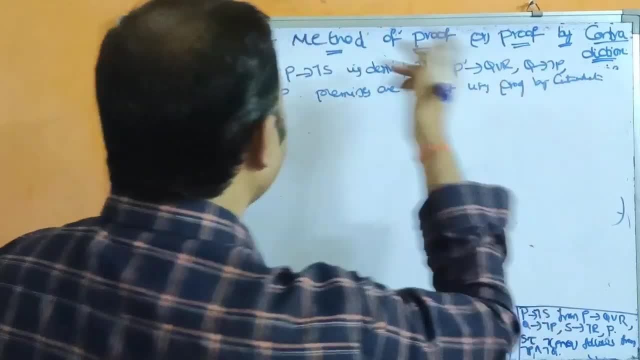 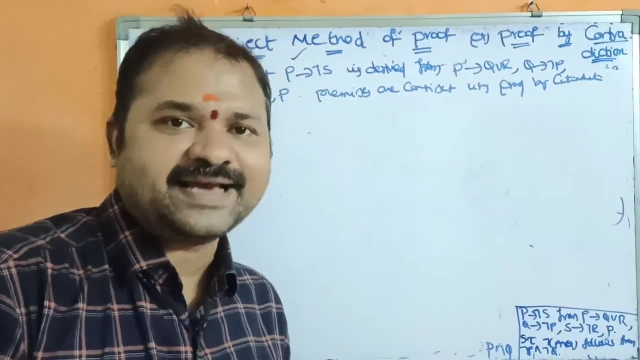 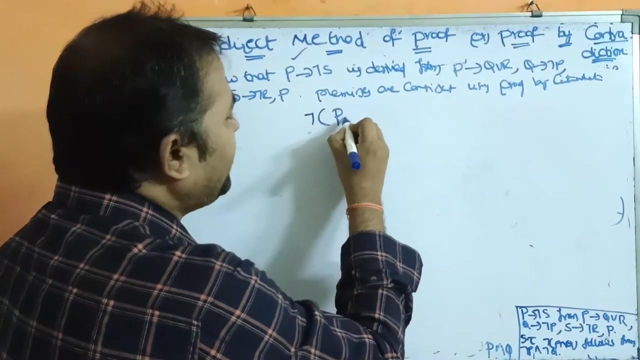 by contradiction is nothing but, uh, this one only, okay, indirect method of proof only show that p implies negation s is derived from that means: p implies negation s is the conclusion here. so what we have to do, we have to negate the conclusion. so negation of p implies negation, yes, so negation of this is in the form of: p implies q. 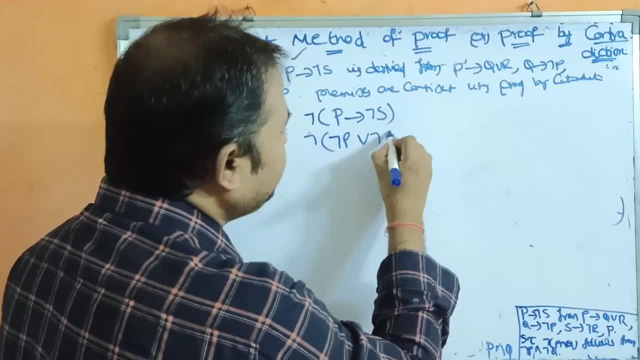 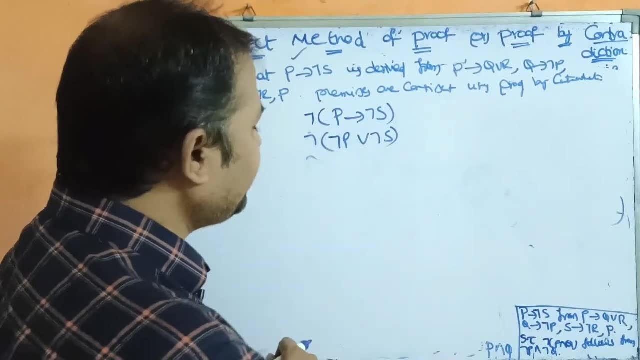 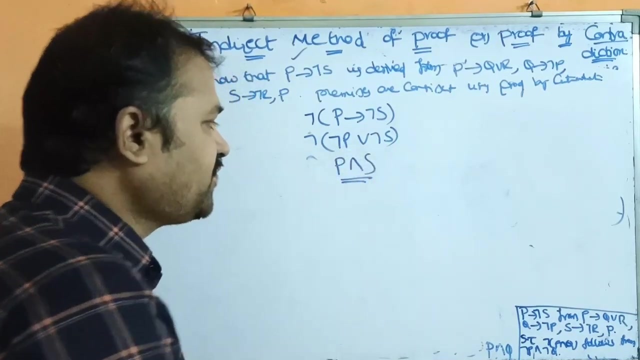 so we can write as negation p? r q. so q means negation s. so negation of this is in the form of p? r weak. negation of exceeding q means what? negation p and negation q. negation of negation p means p, negation of r means, and negation of negation yes means yes. so we got. 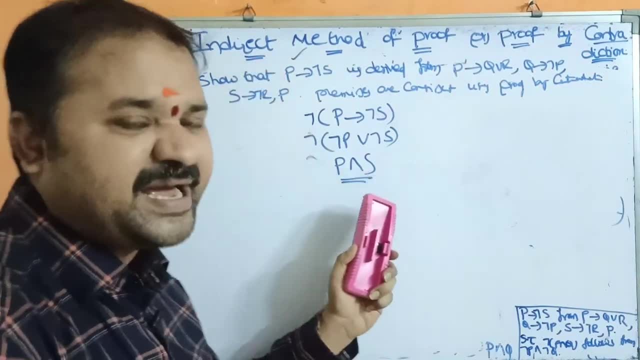 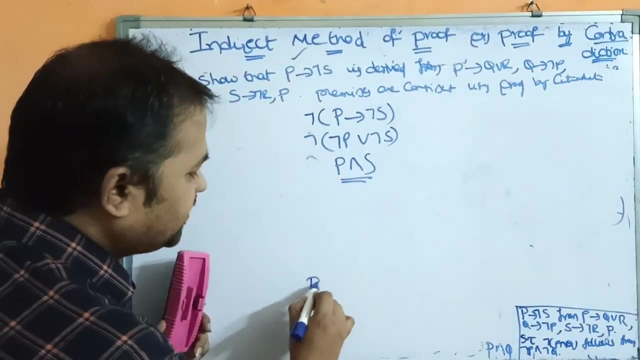 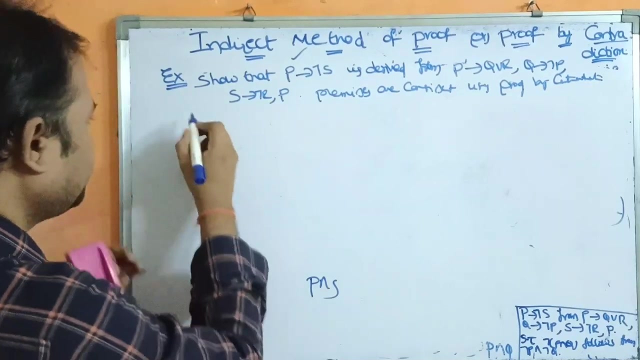 p and s. negation of the conclusion means p and s. so we have to add this new premise to the existing premises. so what is the new premise? p and x negation verbs is nothing but p and s. so for the space constraints, i am erasing this portion. 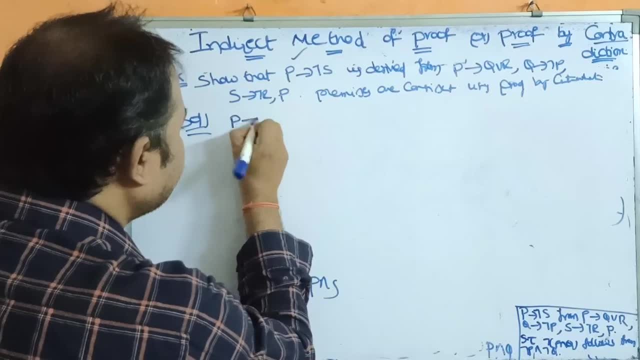 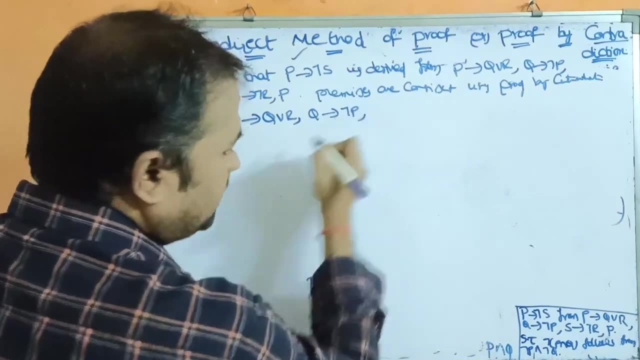 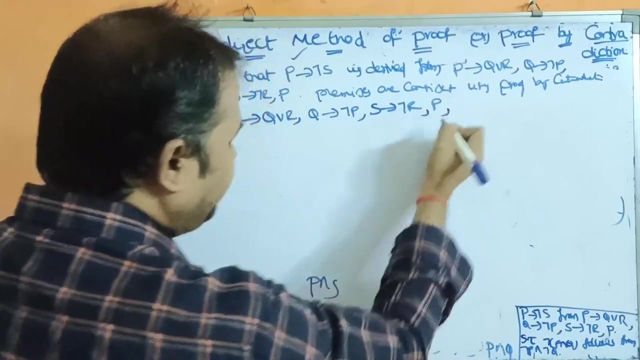 note down the premises here. so the premises are: the first premise is p- conditional q, r, r. the second premise is q- conditional negation p. the third premise is s conditional negation r, s conditional negation r. fourth one is p. and what is the new premise? negation of the conclusion. 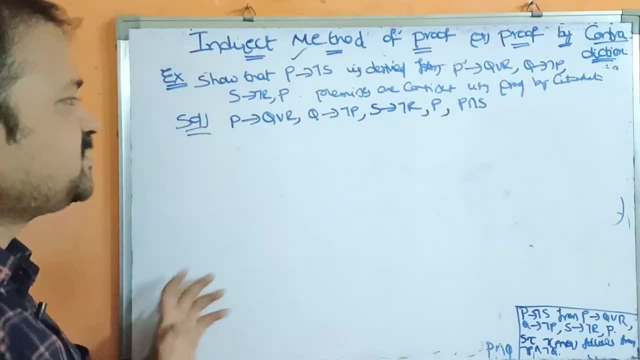 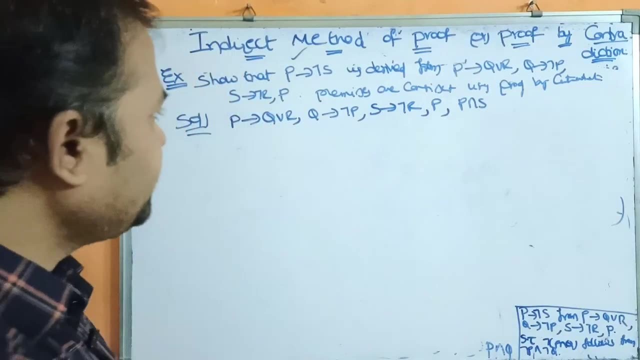 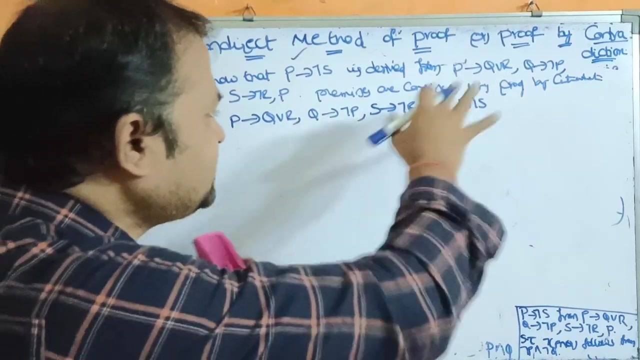 means p and s. so we have to prove that these premises are inconsistent. so that means we have to get the result as contradiction. that is false. okay, if we observe here, first we have to check for the single term premises. why? because here we don't have the, for we here the premises are not in the. 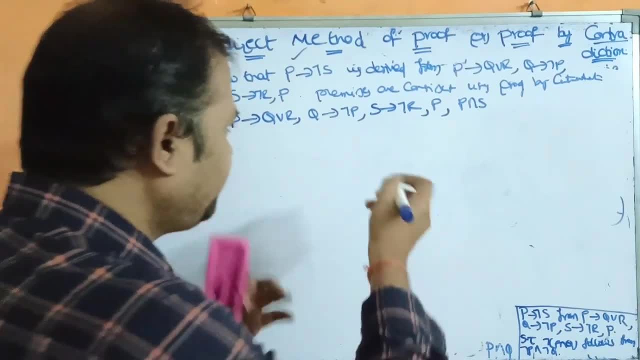 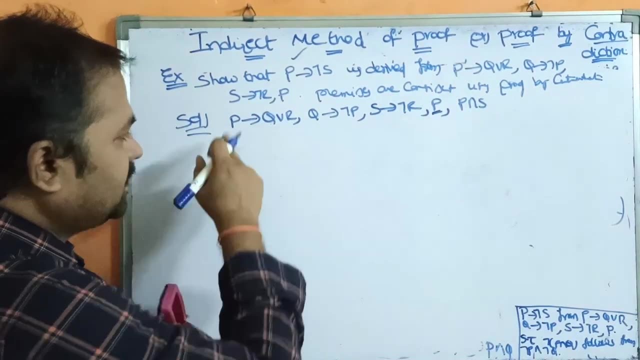 form like p conditional q and q conditional r. okay, if we observe here: here this is the single term premise. so with p we have this premise: p conditional q or r. so we can cancel the p, so we'll get q or r. so let us introduce the first premise. so one formula, number one. 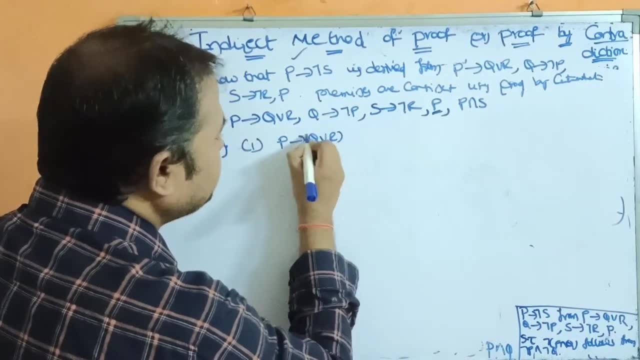 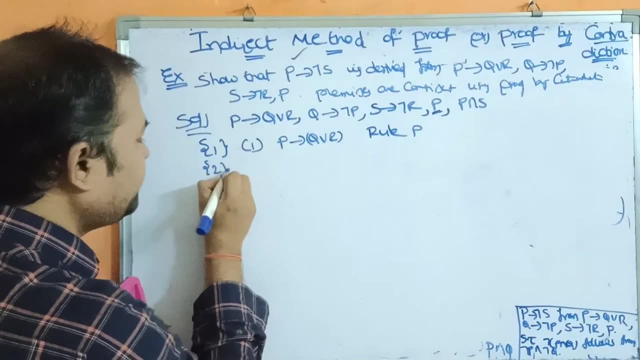 so let us introduce p, conditional, q, r, r. so this is nothing but one statement, right hand statement. so introduction of the premise is nothing but rule p. now let us introduce the second premise, formula number two. so let us introduce this one. okay, this introduction is over this interaction. 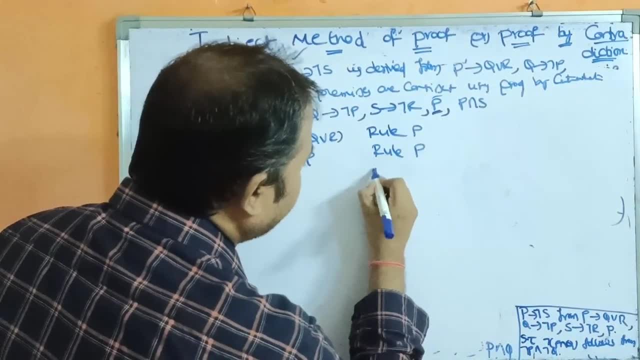 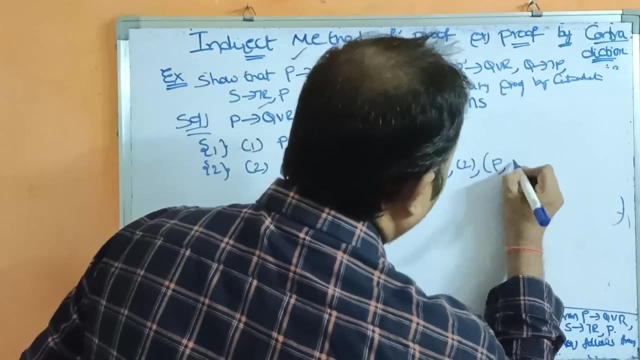 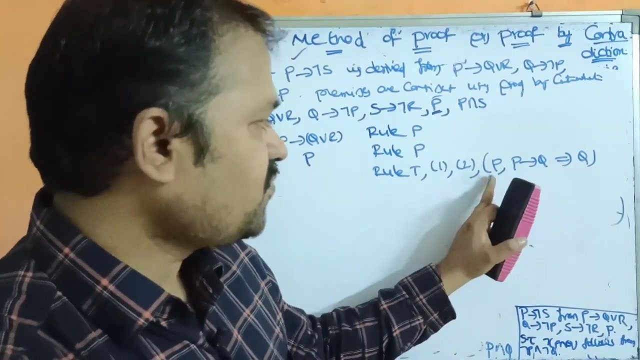 is over. so this is nothing but rule p. now let us apply rule t. rule t on which formula numbers one comma two, one comma two. here we have a formula called p comma. p conditional q implies q. why? because p conditional q means what negation p or q, so we can cancel p and negation p, so we'll. 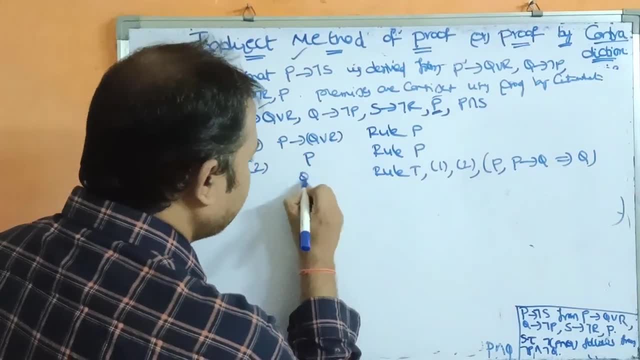 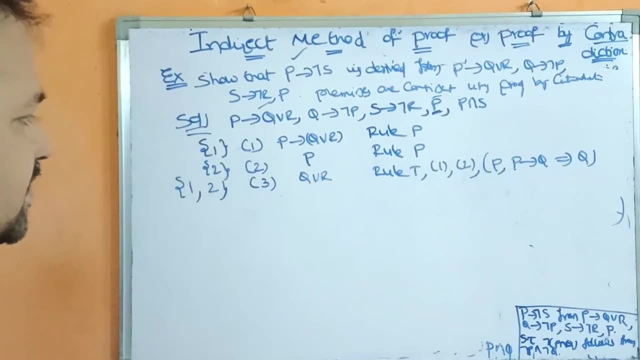 get q as the result here. q means what? q r? q means q r. so the next formula number is three. here we are getting this formula based upon these two premises. so here we have q r r. if we observe here, here also we have q- implies negation p. so let us, let us change this formula into like this: okay, 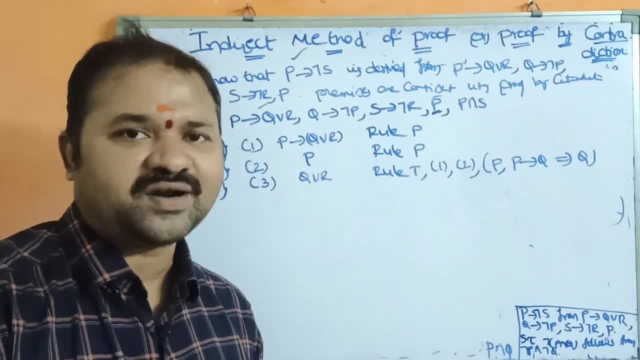 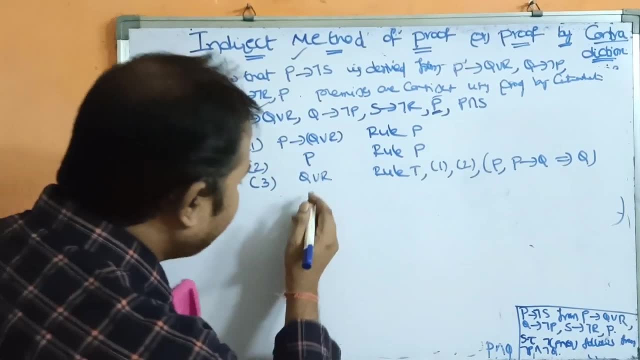 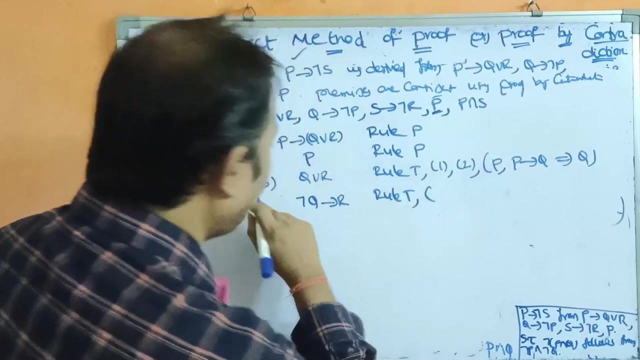 so if we have p, p conditional q, q conditional r, then we can write as p conditional r. okay, here we have a formula called p implies q. means what negation p r q. so we can write this as negation q implies r. why? because here this is nothing but rule t. so on formula number three. so what is the? 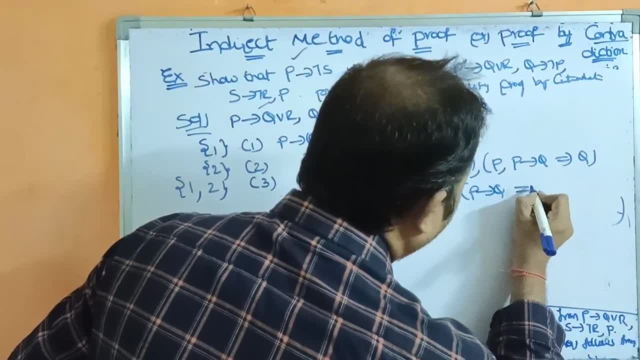 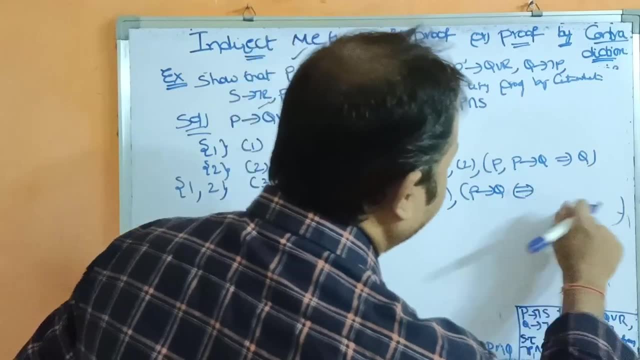 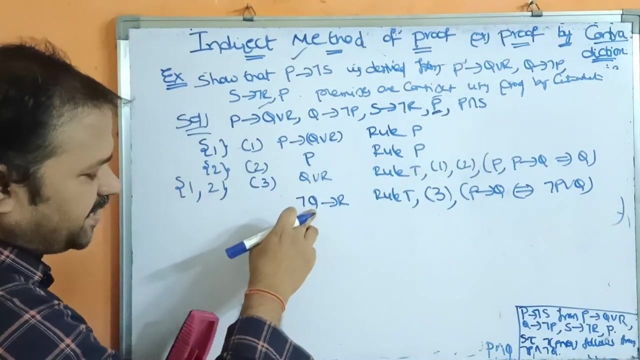 formula we have: p implies q is uh. is uh equivalent to why? because this is nothing but what uh? which? which law? This law is nothing but equivalent law. Negation P R Q. Okay, Here this is nothing but P implies Q, So we can write this as negation P R Q. So negation of negation Q means Q. 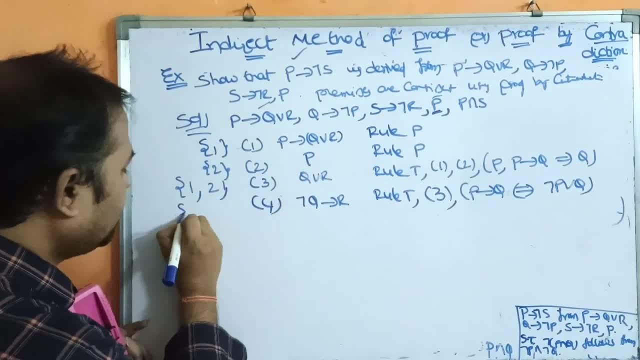 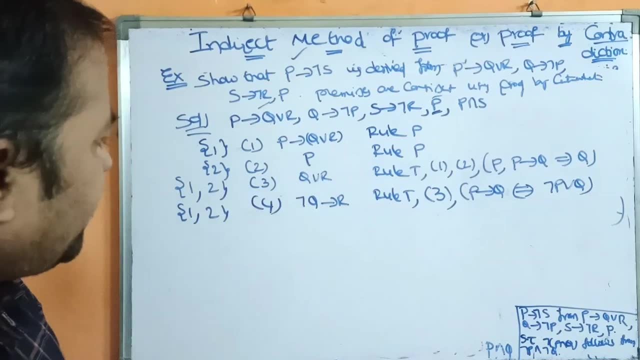 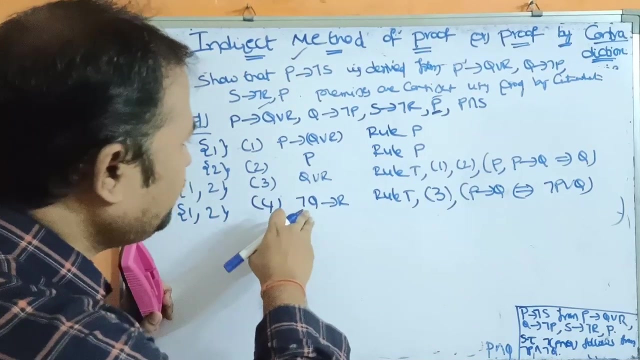 So Q R, R. Okay, So this is nothing but formula number 4.. Here we applied formula on this premise only, Okay. Next, here we have negation Q, conditional R, Various. here we have Q, conditional negation P. So here we need to change this one, So we have to place Q at right hand side. 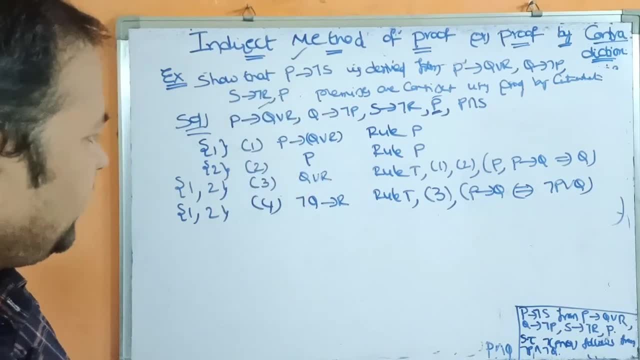 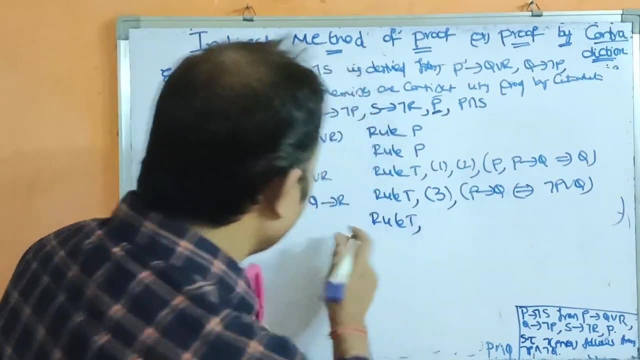 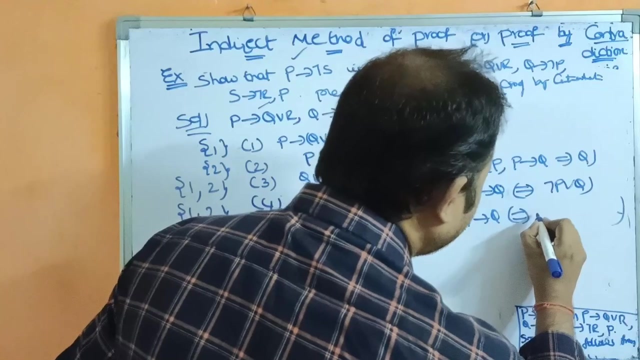 R at left hand side, so that we can apply that formula. Okay, So how we can do that? So here we have a formula called contra positive law, So rule T. Next, here we are applying the formula on 4. We have a formula called P, conditional. Q is logically equivalent to negation, Q implies 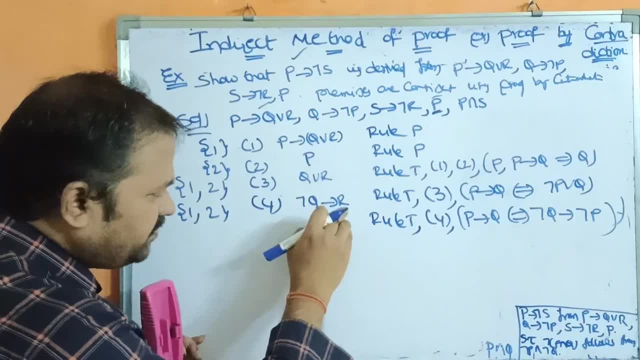 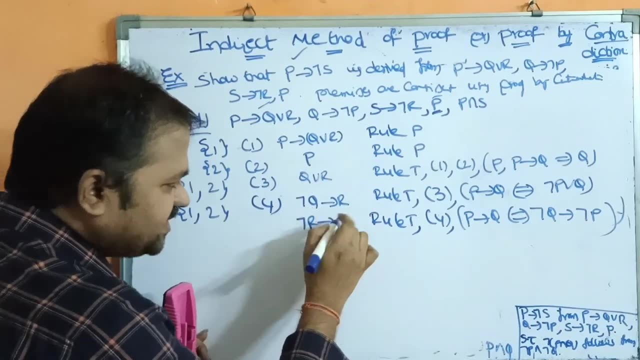 negation P Here. what is negation Q? Negation Q means negation R implies negation P. Negation P means what? Negation of negation Q? Negation of negation Q means what Q? Okay, So this is nothing but formula number 5.. Here we applied. 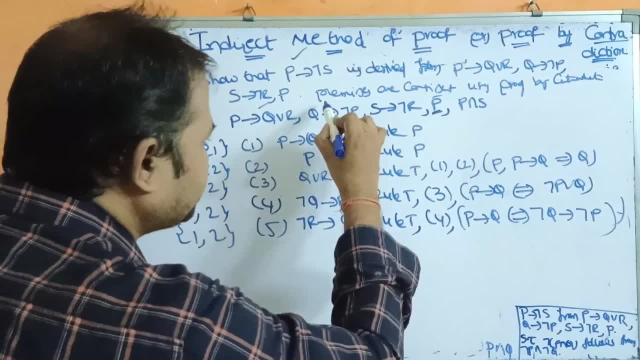 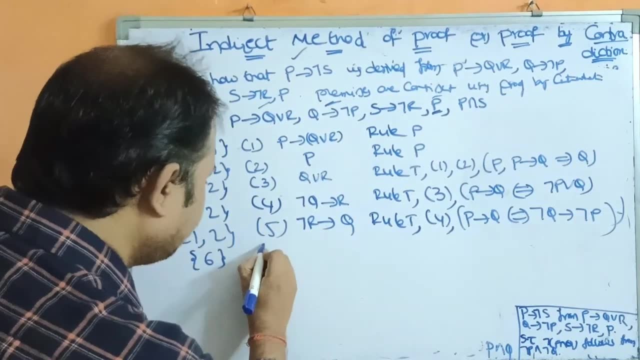 the formula on this premise only. Okay, Now we can introduce this premise: Q, conditional negation, P. So 5 formula number is over. So the next formula number is 6.. 6.. So formula number is 6.. Premise is 6.. Formula is 6.. Let us introduce this premise: Q, conditional negation. 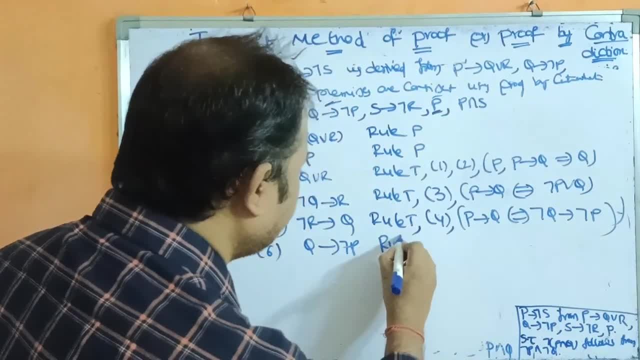 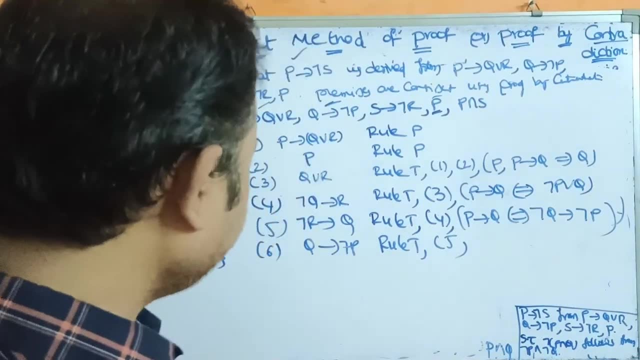 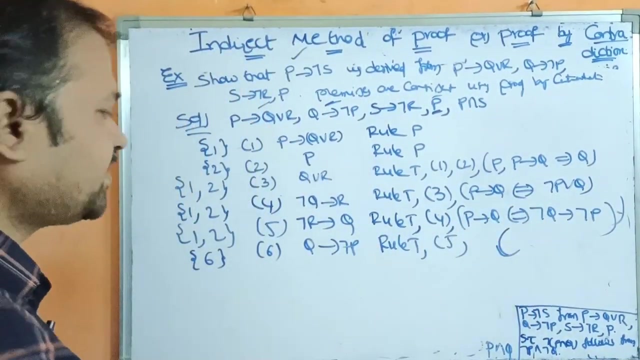 P, Q, conditional Negation: P. So this is nothing but rule T. We applied on which formula number 5. 5. We applied on which formula number? This is nothing but 5.. Okay, And which formula we applied Already. we have written here. So same formula: P, conditional Q means what Negation? 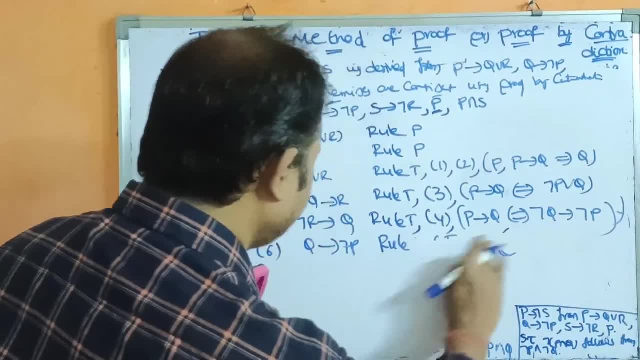 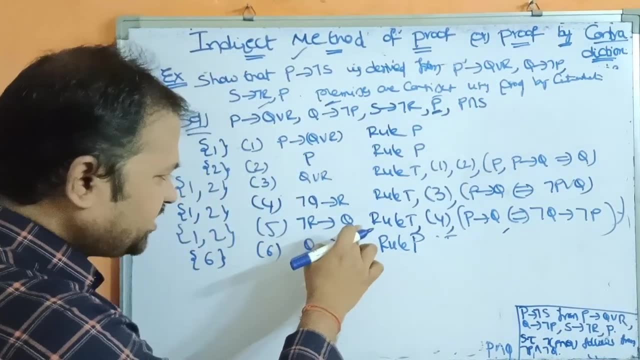 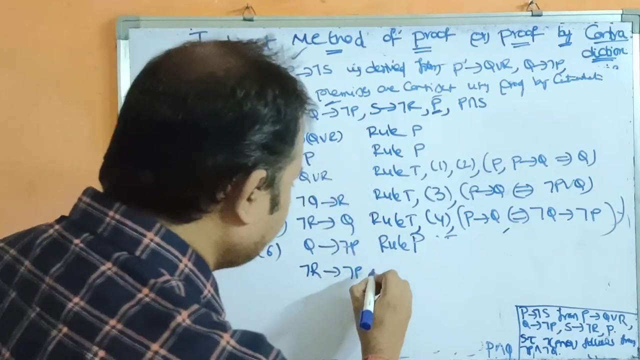 Q. So this is nothing, but I am sorry. So here this is nothing, but introduction of this premise. rule P: Okay, Now here this is in the form of P conditional Q, Q conditional R, So we can write here as P conditional R. So negation R implies negation P. Here this is nothing. 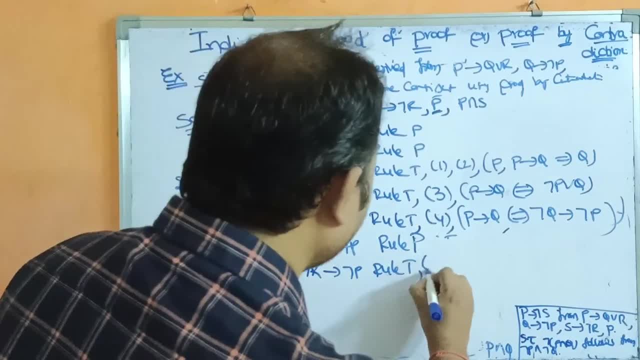 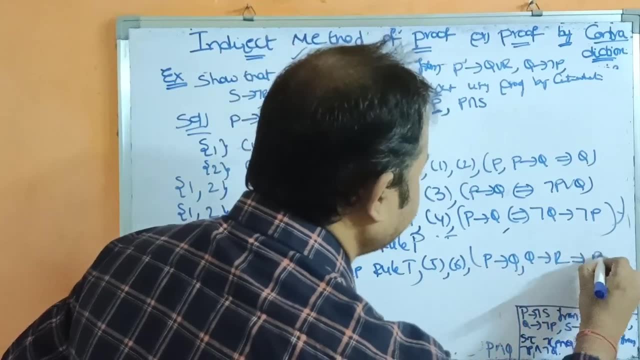 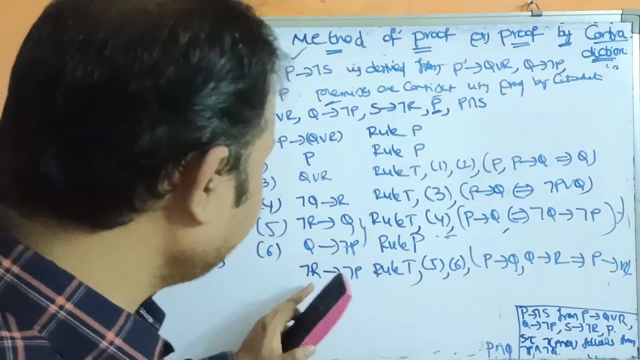 but rule T We applied, on which formula numbers, So 5 and 6.. And the formula here is: P conditional Q comma: Q conditional R implies P conditional R. So from these we are getting this premise: Negation R implies Q, Q conditional R, negation P means what Negation R implies negation. 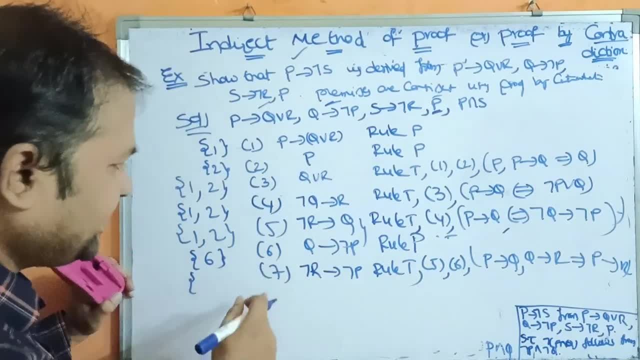 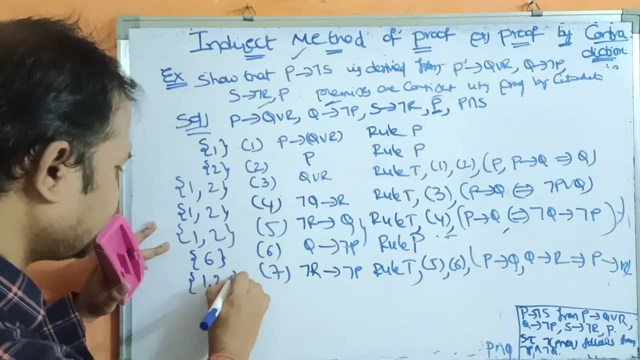 P. So this is nothing but seventh formula number. And what is this premise? This is so. this premise is nothing but here we applied on these two premises, So 1 comma, 2 comma 6.. So from these two only we are getting this premise. Okay, So here we have negation R. 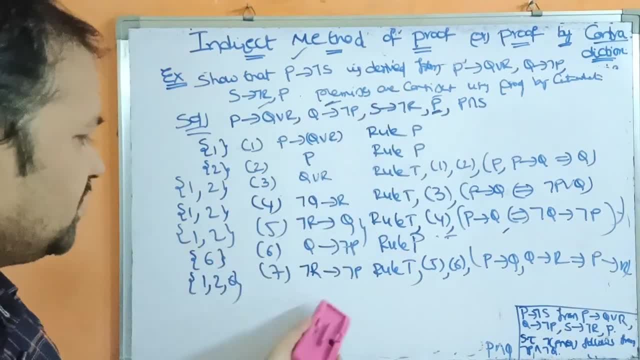 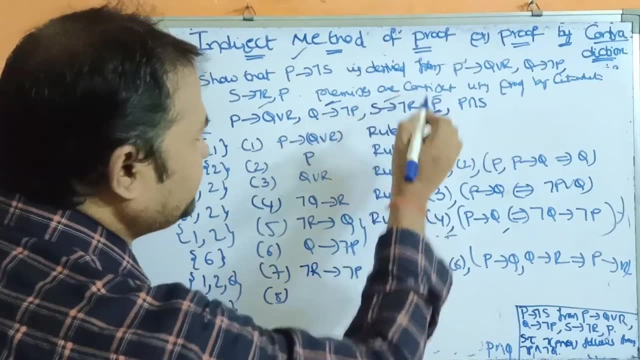 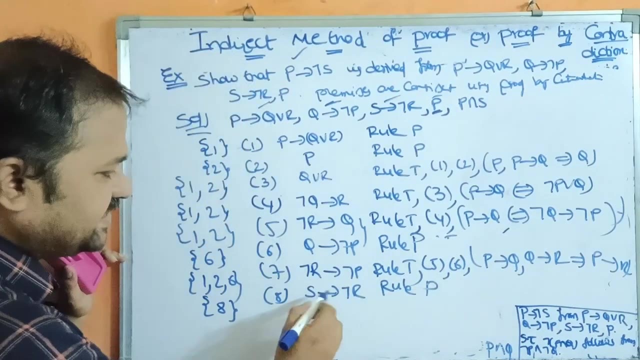 conditional negation P. Here we have S conditional negation R, So directly we can apply the formula. So the next premise: number is 7 is over 8.. Formula number is 8.. So let us introduce the next premise, S conditional negation R. So this is nothing, but rule P. So this is nothing. 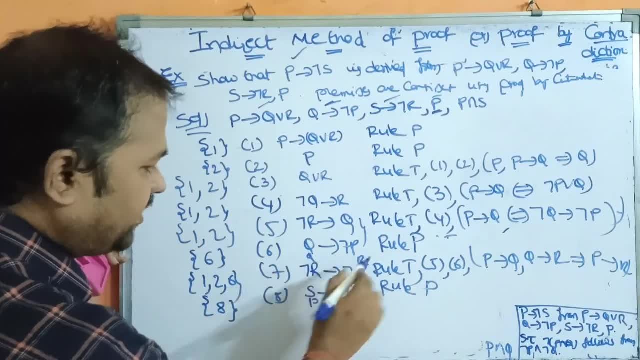 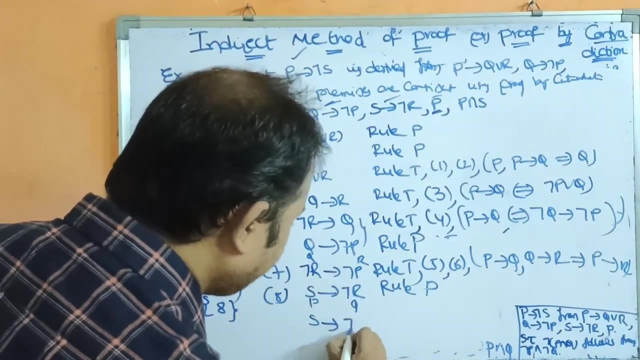 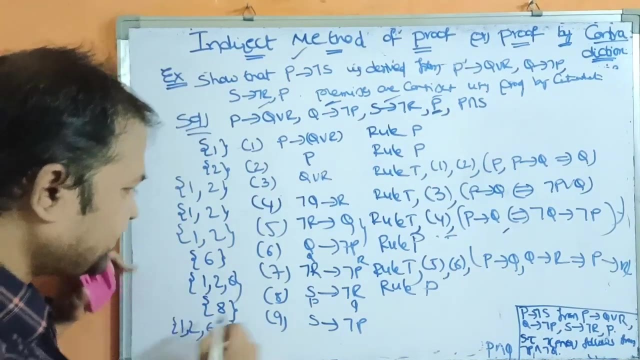 but S conditional negation P. So we can convert this one into what? P conditional R, So S conditional negation P. So this is nothing but formula number 9.. Here we are getting that premise based upon 1,, 2,, 6, 8.. So this is nothing but rule T, on which formula numbers? 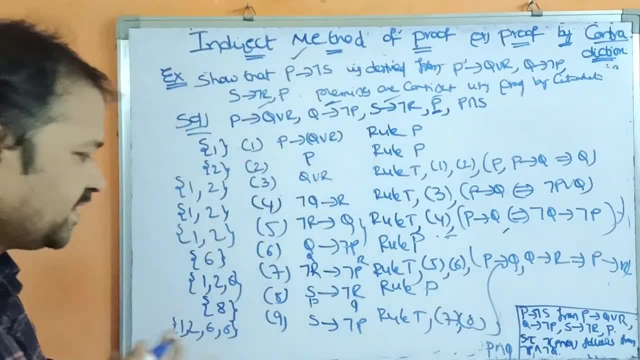 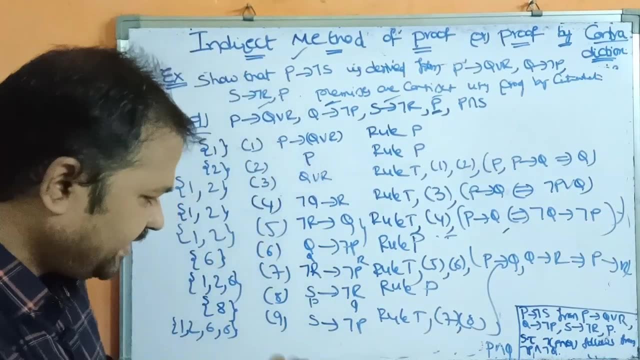 7 and 8.. And this one same formula. Okay. Next, here we have S conditional negation P. So what is the formula for S conditional negation P Here for space constraints? I am not writing the formulas here: S conditional negation P. 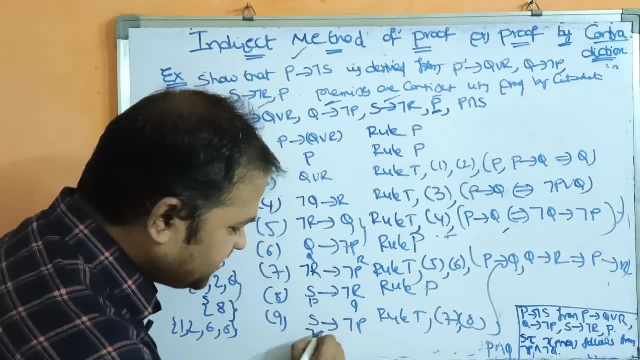 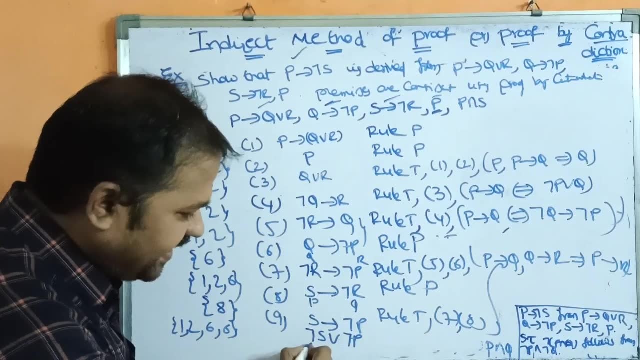 This is in the form of P condition Q, So we can write as negation P R Q. So negation S R, negation P. So this is in the form of negation S R negation P, So we can write this as negation P R negation. 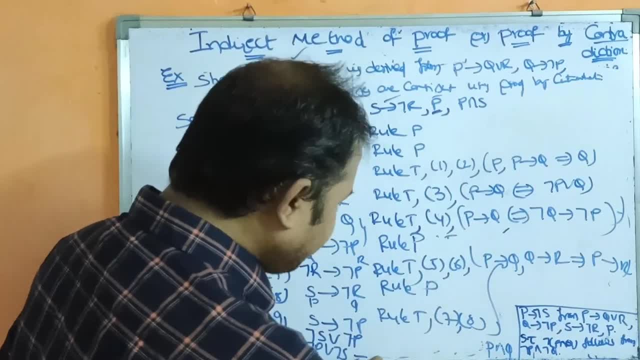 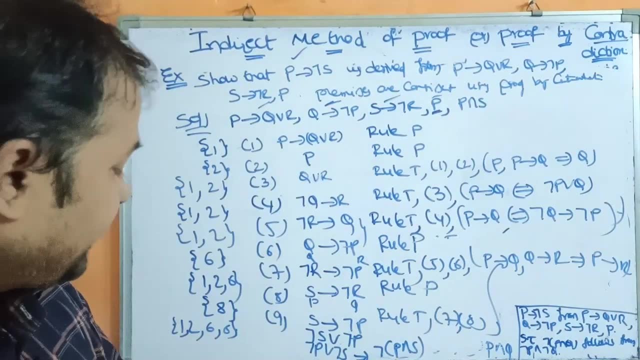 S. So negation P, R, negation S means we can write as negation of P and S, Negation of P and X. Okay, So here we have a premise called negation of P and S. Okay, So from this premise we got: 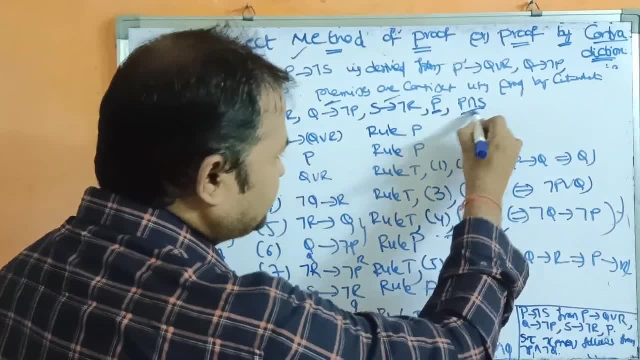 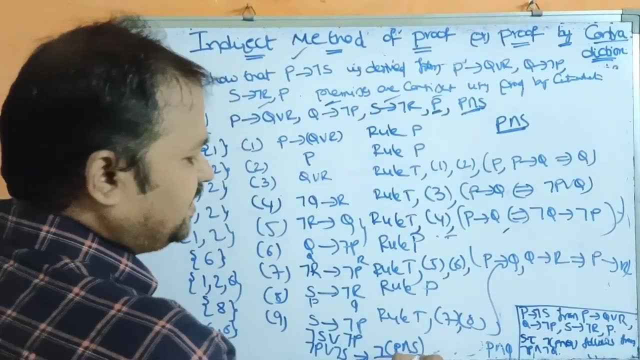 this premise: Negation of P and S. So next we have one more premise, That is P and S. So let us introduce that premise: P and S. Here we have P and S, Here we have negation of P and S. Let it be P, Let it be P. Okay, Negation P. So it will become P. So P and S, and and. 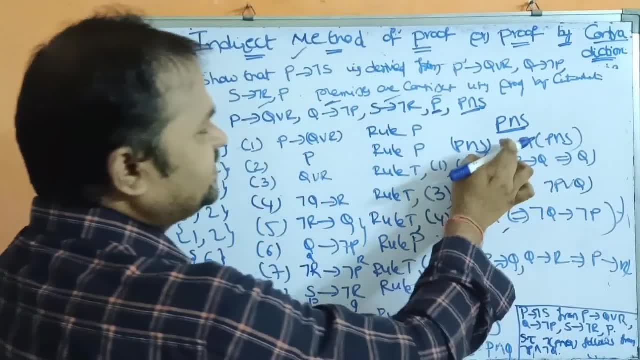 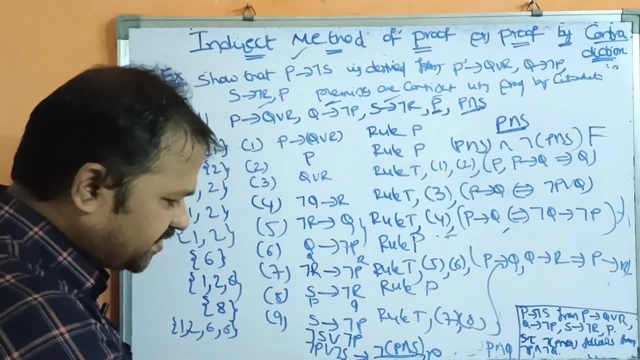 negation of P and S means what? So this is nothing but contradiction. So this is in the form of P and negation P, So the result is false. Okay, In the examination you have to write the formula for these two statements also. 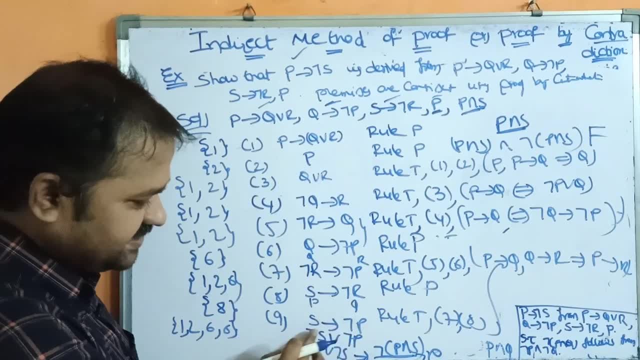 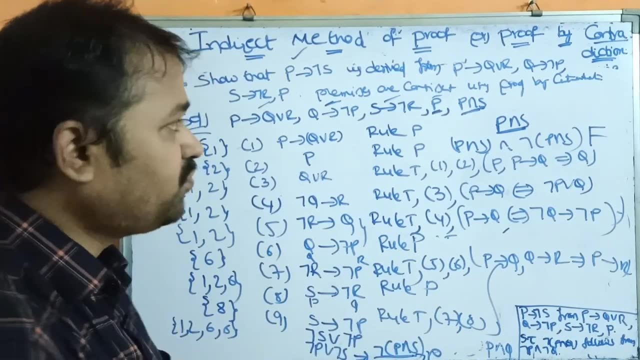 These constraints. I didn't write those statements, So we can write this as negation S R negation P. We can write this as we have committed: EULA: P R Q is implied logically equivalent to Q R P. Why? Because here we have P R S, So that's why we changed the order: Negation P- R negation. 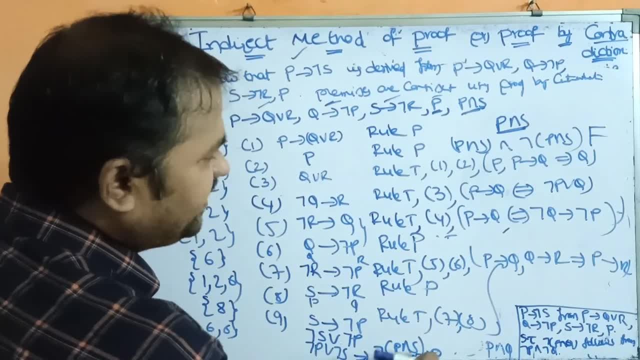 S. We can write it as negation of P and S. So this is in the form of negation P. This is in the form of P. This is the new premise. So P and negation P means false. So we can. 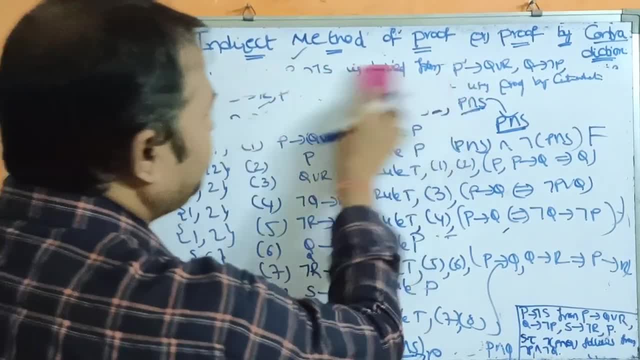 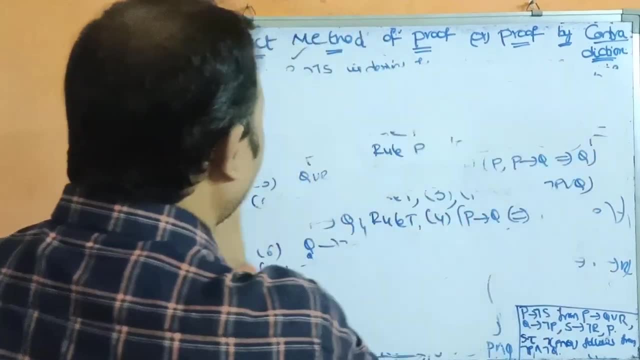 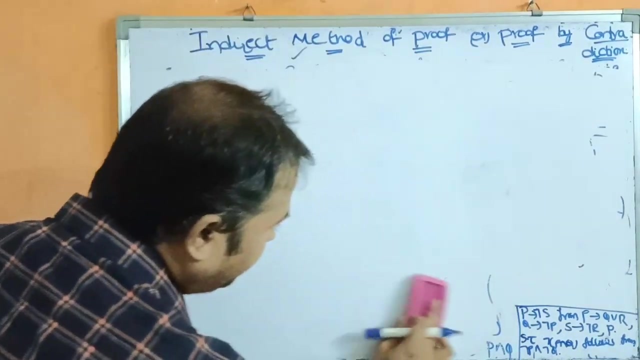 say that all these premises are consistent. inconsistent Why? Because we got the result as false. So if we get the result as false, then we can say that those premises are inconsistent. Now let us see the last example. So this example was taken from Tremblay and Manoeuvre textbook. 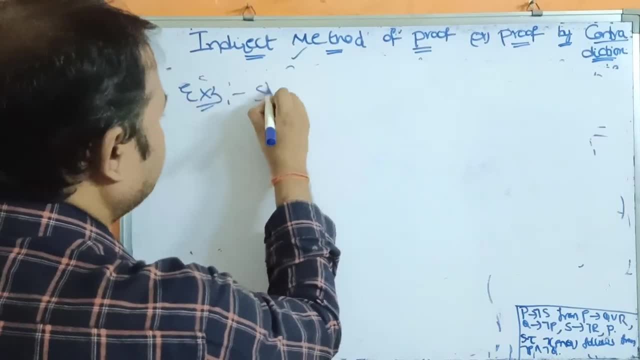 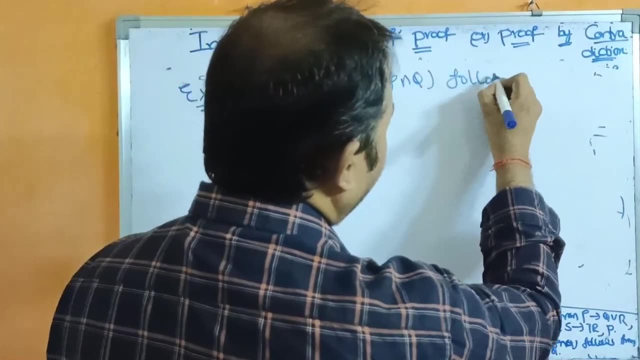 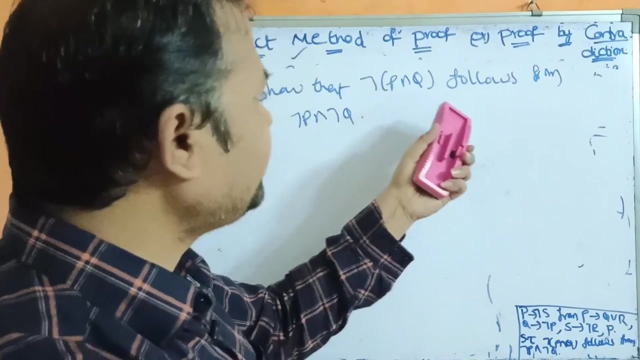 So this example is very, very important example. Show that show that negation of P and Q follows from follows from negation P and negation Q. Okay, show that negation of p and q follows from negation p and negation q. So here this is. 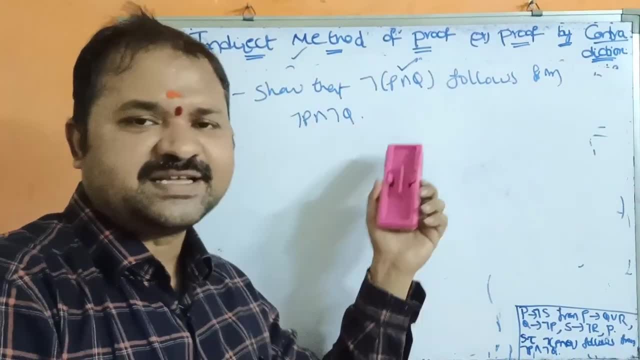 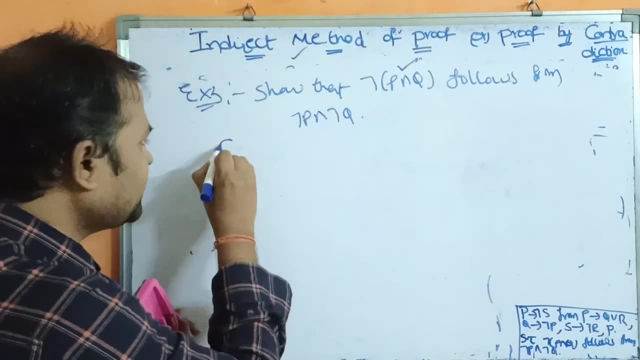 nothing but the conclusion and only one premise is given, that is nothing but negation and p and negation q. So we have to show that with the help of the indirect method of proof. So what is indirect method of proof? We have to calculate negation of the conclusion. So negation of. 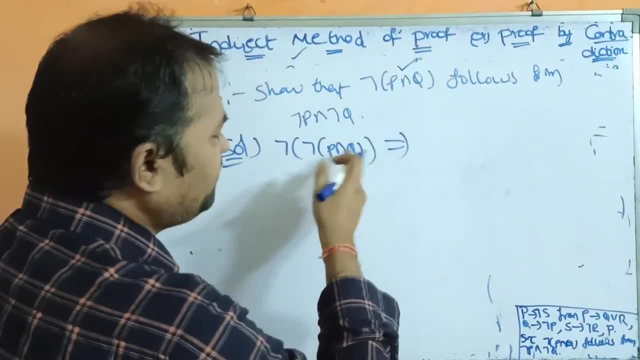 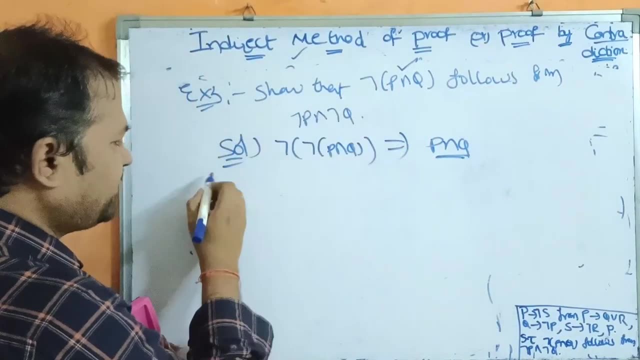 negation of p and q. This is the conclusion. So negation of negation. p means what p, So here p means what p and q. So this is the negation of the conclusion. So this is the. 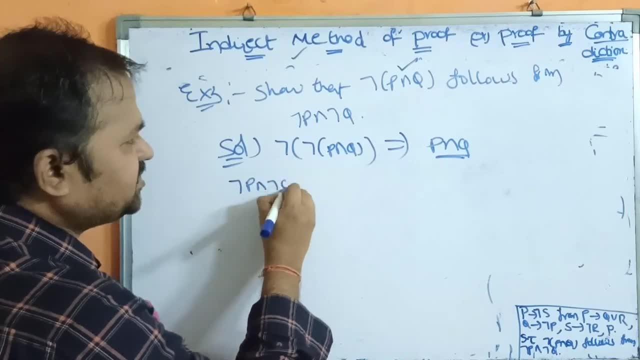 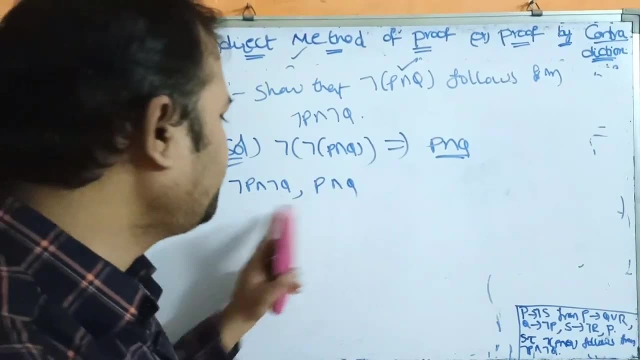 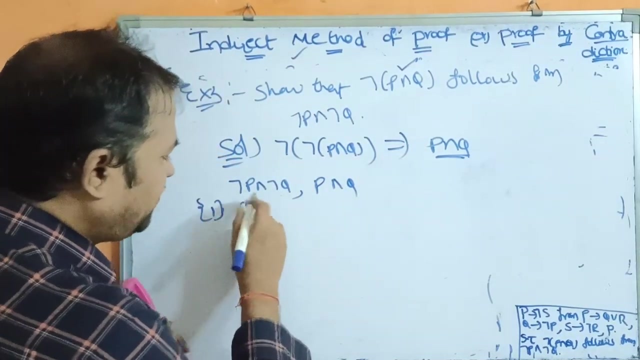 premise. So what are the premises now? So negation p and negation q. So this is one premise, And what is the new premise? p and q. So from these two premises we have to show the contradiction. So let us do how we can write that. So first premise, first formula. Let us 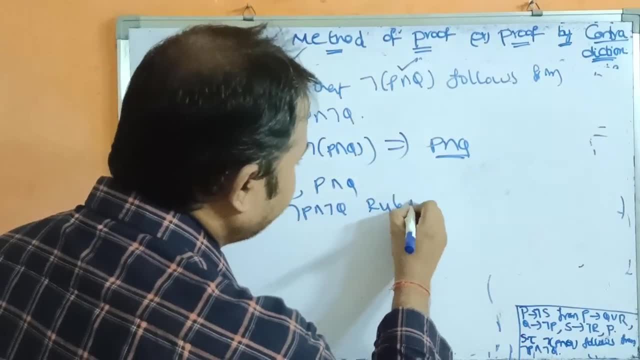 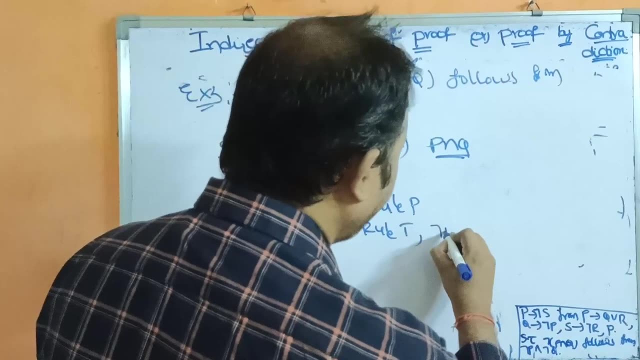 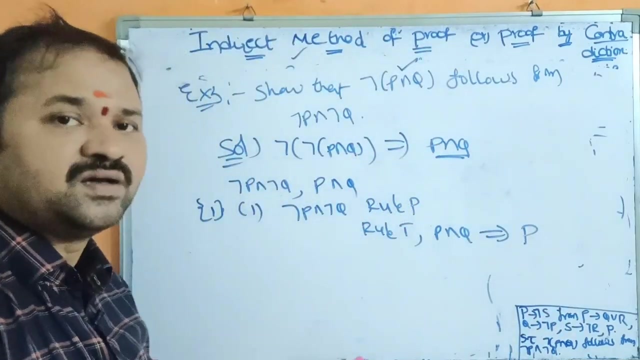 introduce the first one: negation p and negation q. Introduction means rule p. Next let us apply rule t On this premise. So here we have a formula called negation p and q. p and q is implied p, p and q implied p. If we want, we can take q also. So here p means negation p, q means